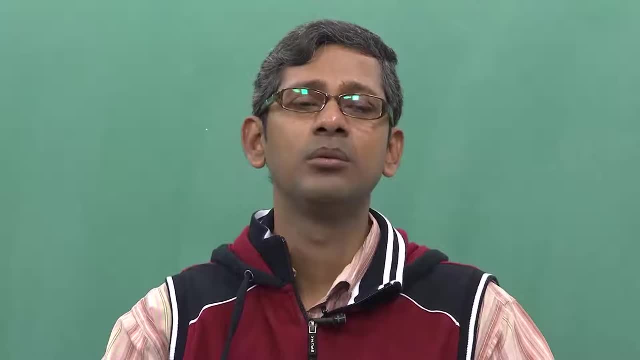 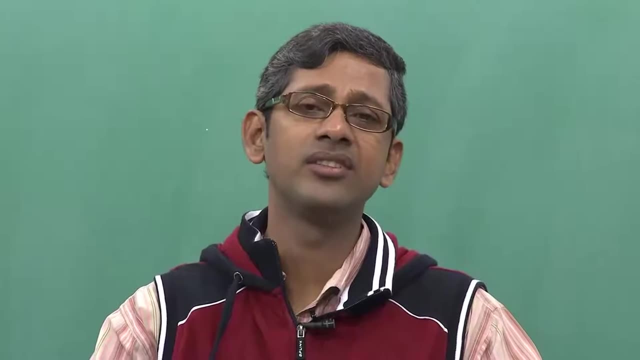 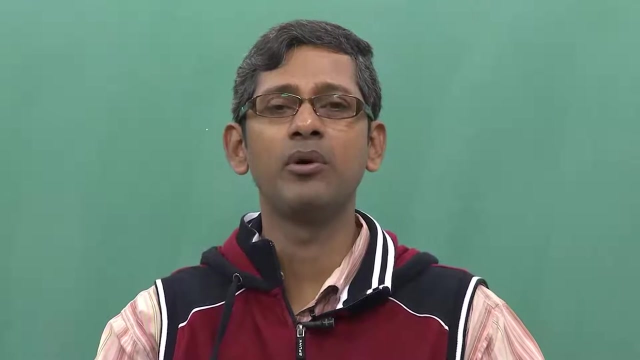 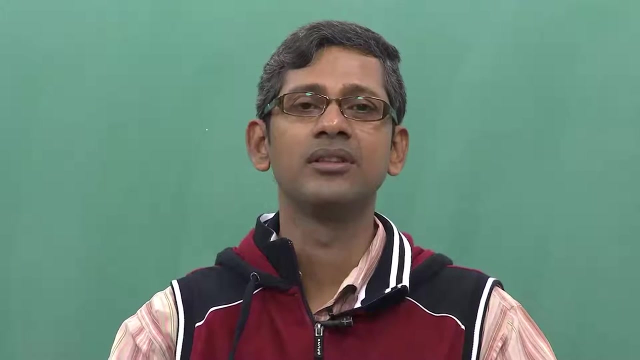 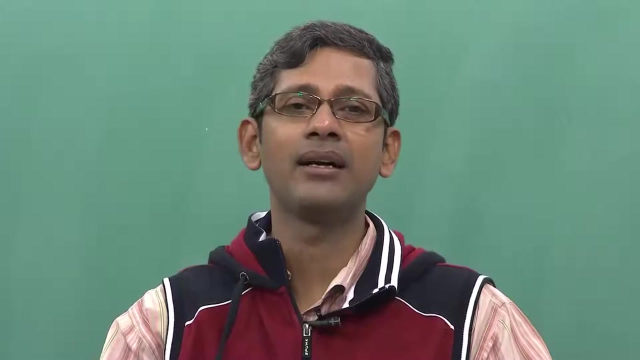 inside the furnace. and then at the end of Friday, before he was going out for weekends, he hurriedly opened the furnace and mistakenly one sample came out from the furnace and fell onto a bucket full of water. So he did not look into it, He just ran away, and next week, on Monday, he came back. 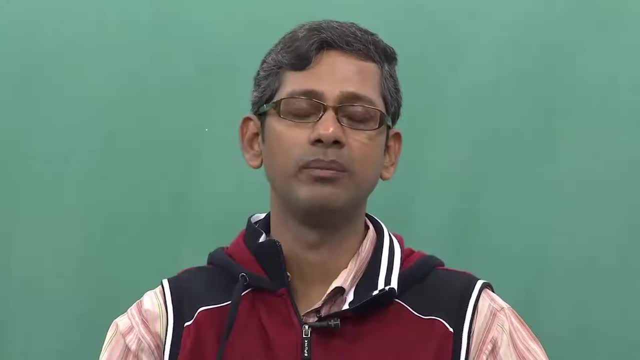 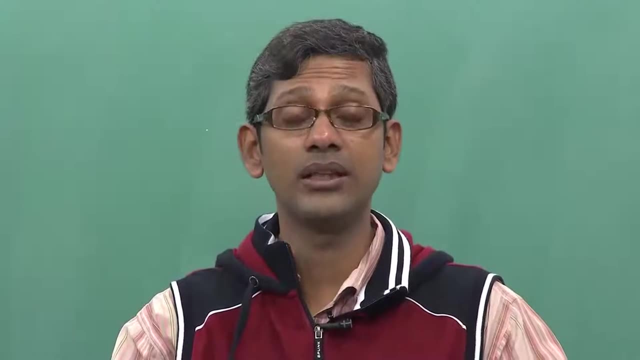 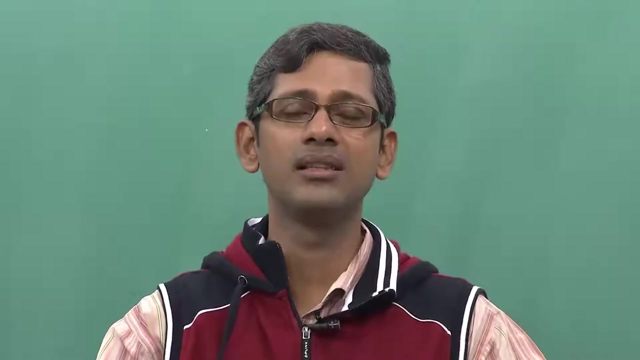 and he just saw the sample which is inside that bucket full of water. Then what happened? He was an inkling guy. Although he was working on pearlitic affirmations, he did not throw this sample away. We will think: what is there in a sample? Let me just throw it away because 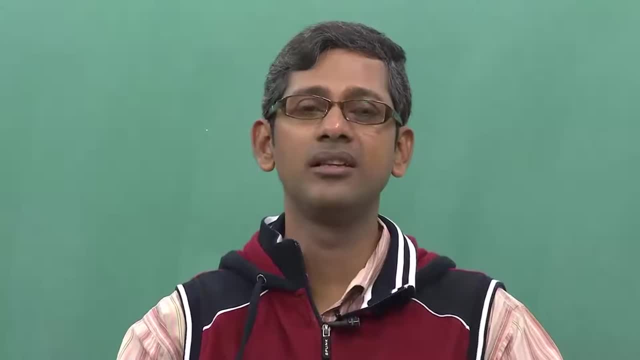 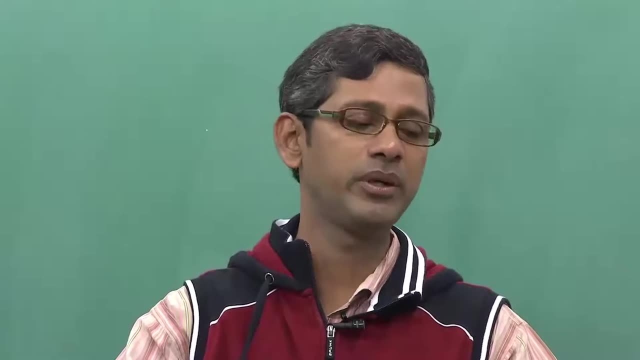 will happen if I quench steel in water. but this fellow was intelligent. He took out the sample first thing he saw. the sample was very hard. that you can see from the sample. You can take a nail and make a scratch on the sample. it was not. 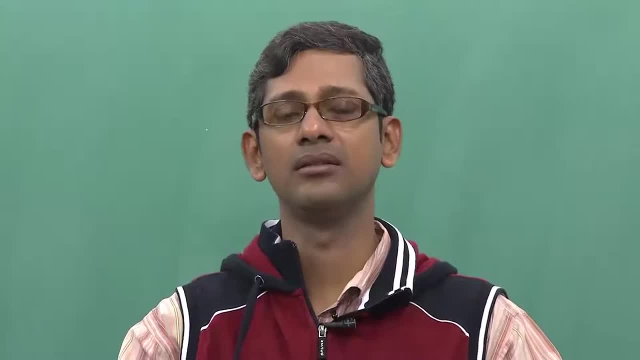 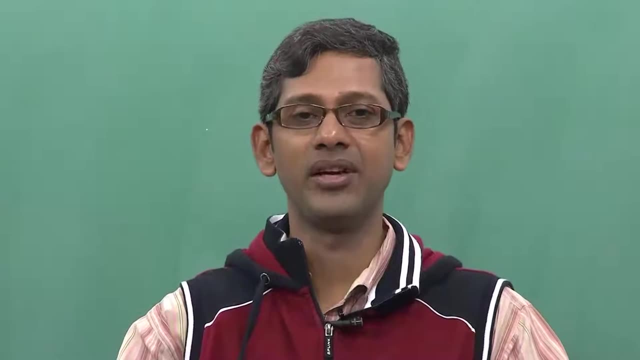 So he went and measured the hardness of the sample and it was very hard. It was much, much harder than the normal pearlitic sample. and then he went on discovering what is martensite, and the whole phase which he discovered he named after his name. that 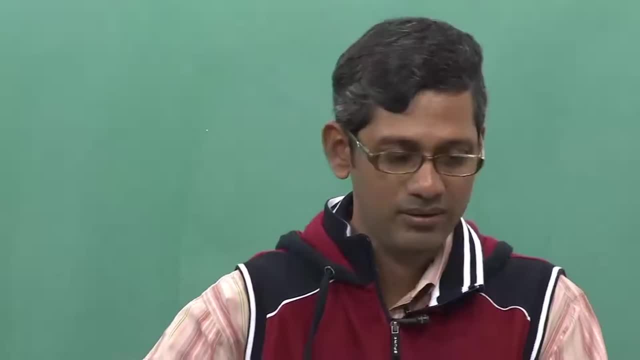 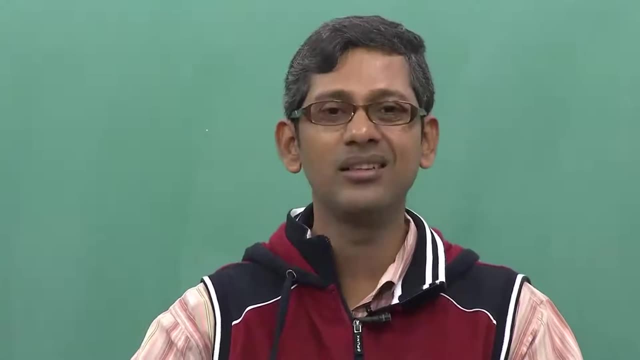 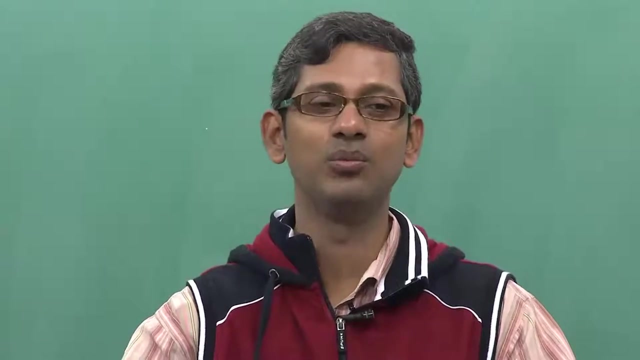 is called martensite. So the moral of the story is that in your experiment, if you do something which is unusual, which you think is not important to you, please do not throw it away. You must judge it, you must investigate it and you may find interesting stuff like this: 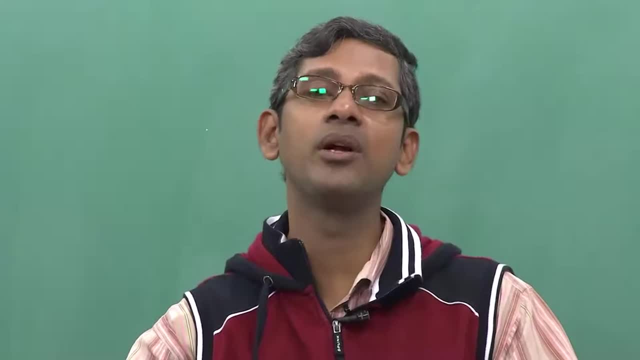 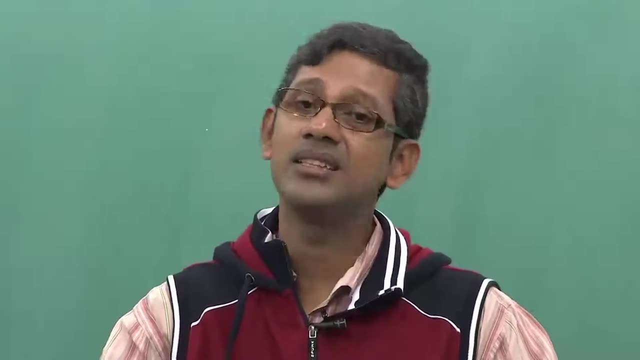 and you may be immortal. We call it martensite or martens because everybody will say the name martensite, they are calling the name of martens. So that is what actually happens. Now you know martensite is a separate phase in steel. it is not a pearlite like mixer. 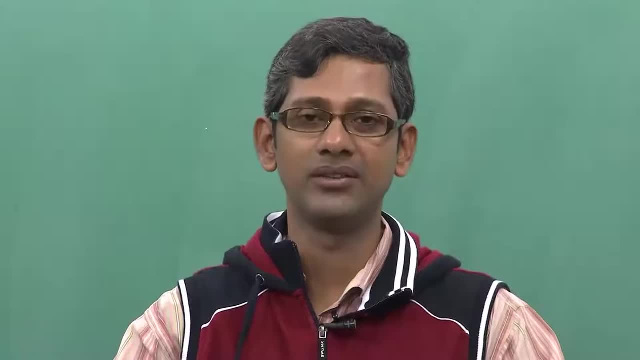 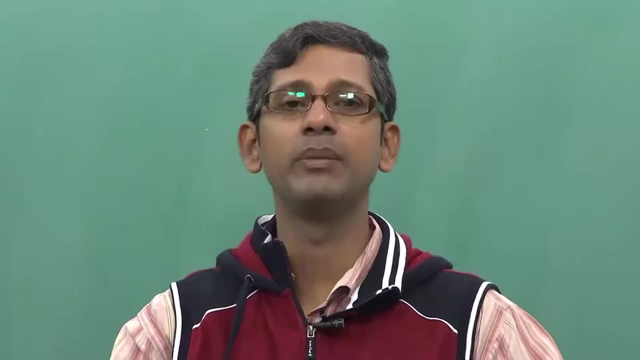 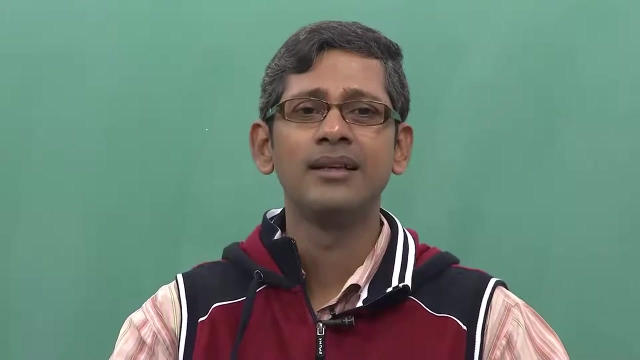 of two phases and martensite is a very important phase. What will happen? as I discussed about pearlite transformations, pearlite transformation depends on what Depends on, basically, the diffusion of carbon, The carbon in gamma Rn. The carbon in gamma Rn has to partition between alpha and cementite. then only pearlite can. 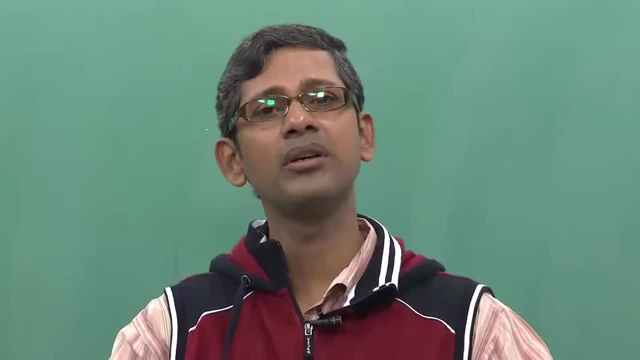 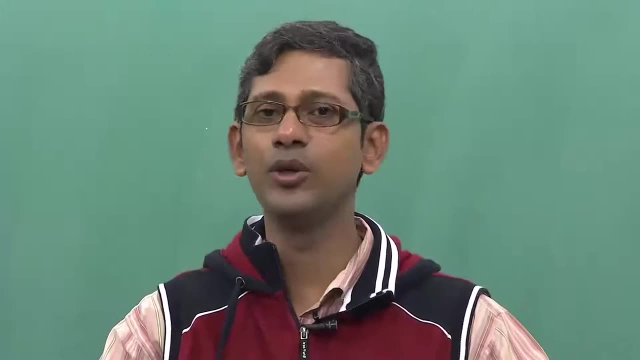 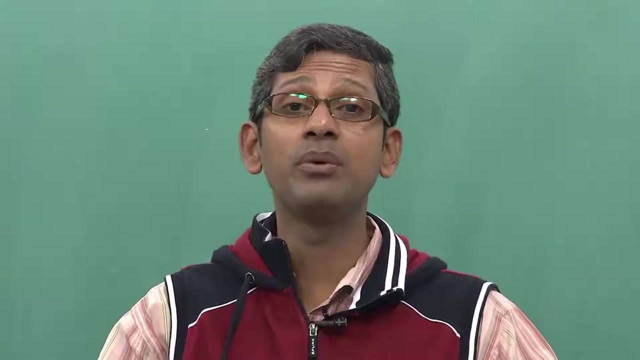 form, because cementite contains large amount of carbon, alpha Rn does not contain, and they will form like a lamellar morphology which I have been drawing you in the last few classes and you have got an idea about it, how to draw it. So this partitioning of carbon will be dependent on the diffusion of carbon. 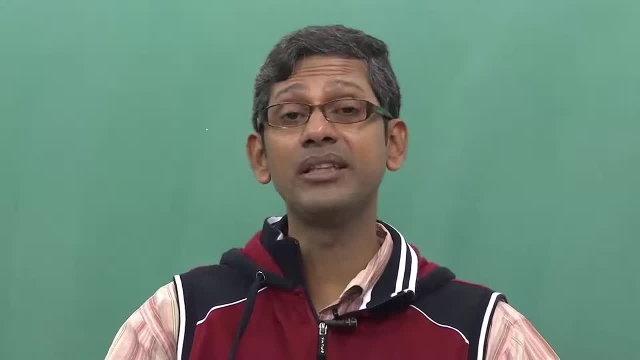 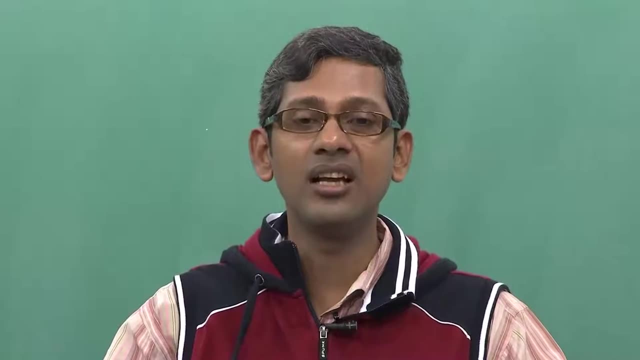 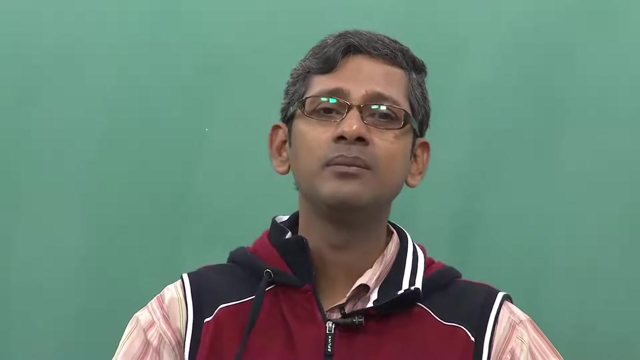 So now the question is that diffusion of carbon is a time dependent process. although diffusion of carbon is very high at high temperatures, because it is interstitial, but it is not infinite. It has certain value. So if I do an experiment in which I drop the temperature of sample from 950 to room temperature, 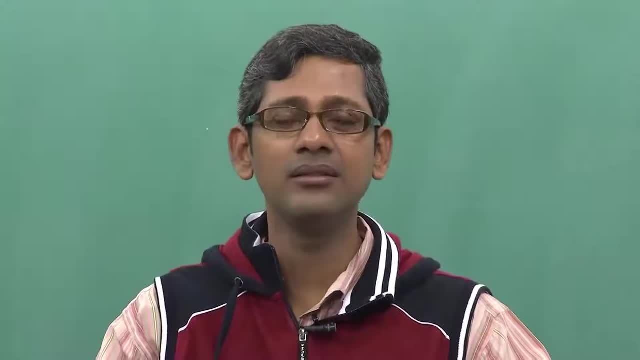 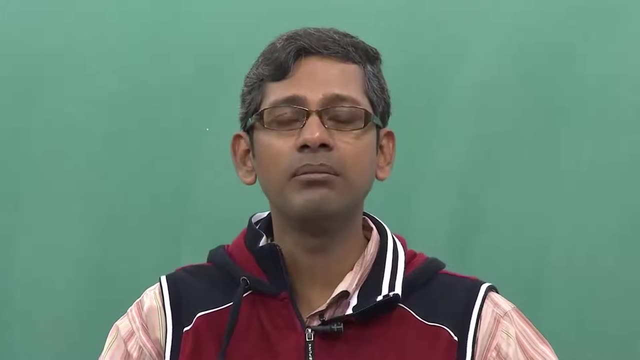 in couple of seconds, just like what martens has done. then what will happen? diffusion of carbon is no longer possible because diffusion requires certain amount of time. You are not giving a certain amount of time. You are not giving a certain amount of time. 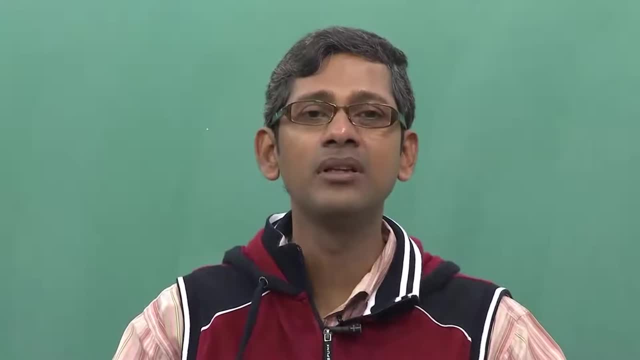 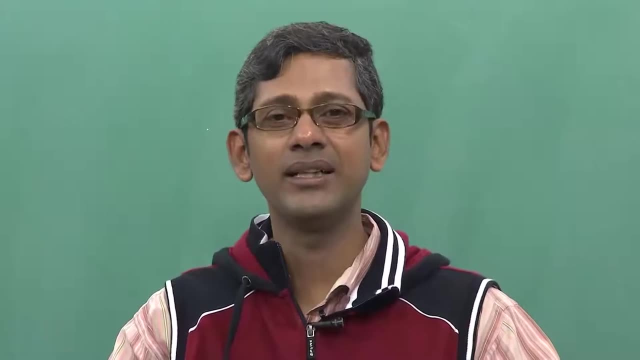 You are not giving a certain amount of time, You are not giving the time, You are taking the sample at 950 Celsius temperature and directly putting into water. That means by that you are bringing the temperature sample from 950 to room temperature in couple. 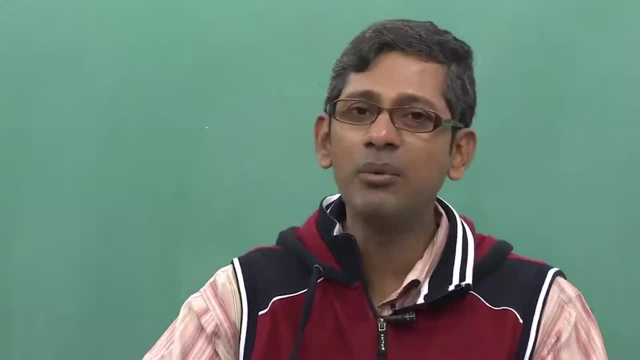 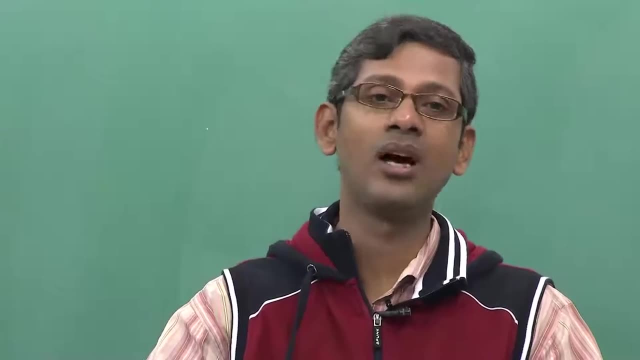 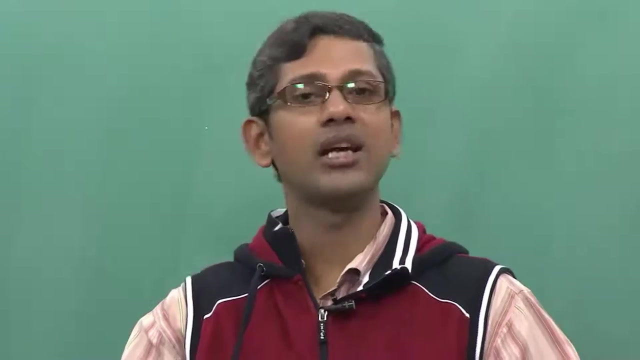 of seconds or within few seconds. So because carbon cannot diffuse what will happen. But gamma will remain gamma. Do you think so? Answer is no, because gamma is not stable at room temperature. Carbon is only stable at high temperature. So gamma has to transform something, and that something is known as martensite. 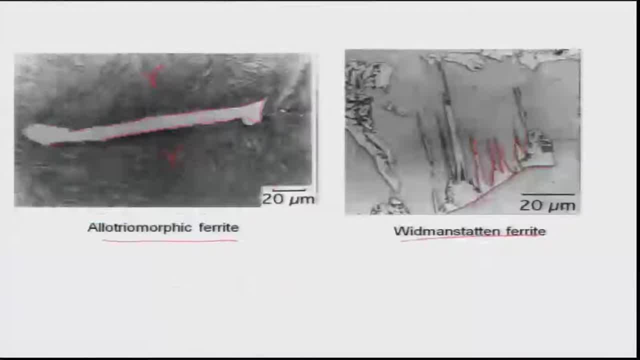 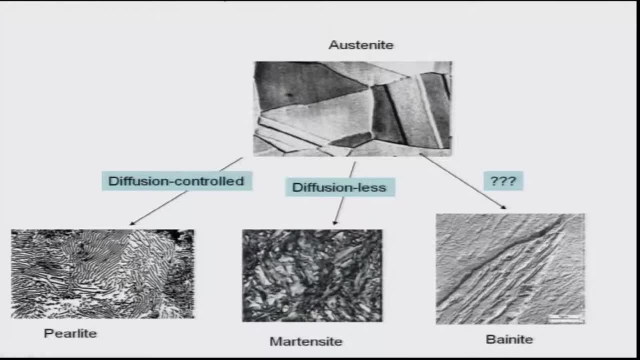 So important thing is that what I showed you at the beginning- I will go back in the slide- Important thing is that martensite is a diffusion-less transformation. That is what I have shown you here in this picture. You see here, this is a diffusion-less transformation. 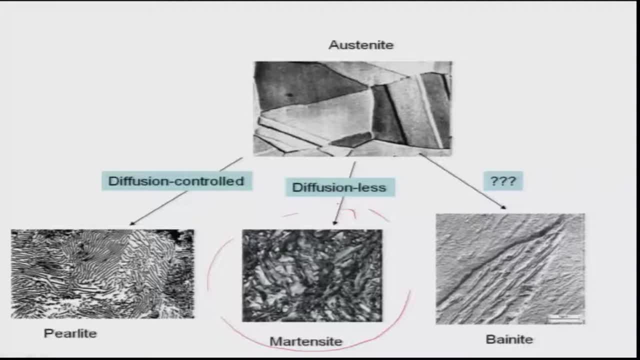 So that means diffusion of carbon is not going to take place or not going to happen. It is not going to dominate the mechanism of formation of martensite. So martensite is a diffusion-less transformation, or it is also known as: martensite is also. 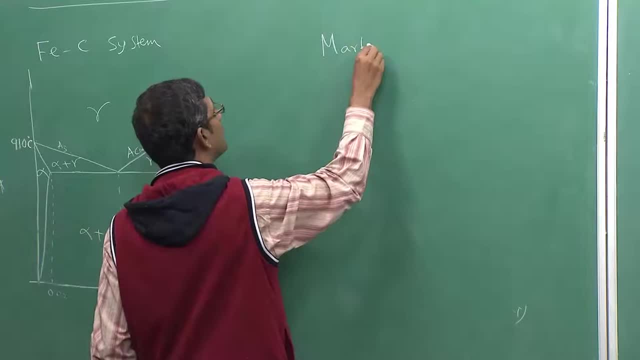 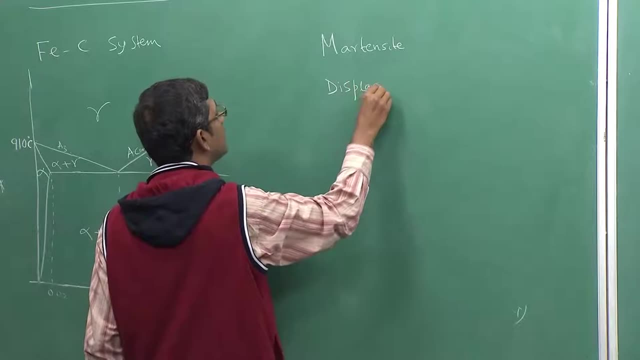 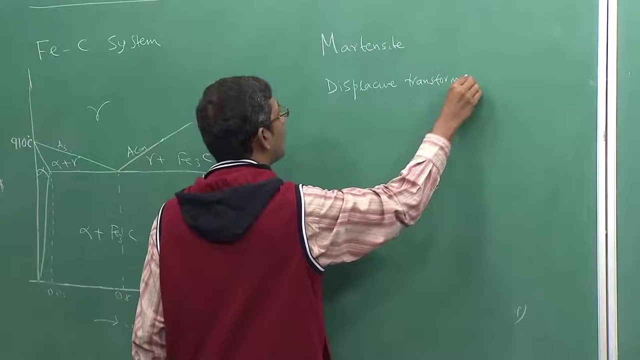 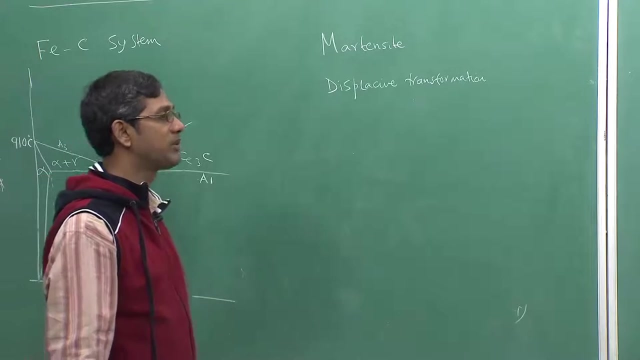 known as displacive transformation. It is also known as a displacive transformation. I will tell you why. Why, Why It is named after the discoverer Martens. It is a displacive transformation, or diffusion-less transformation, as I told you. 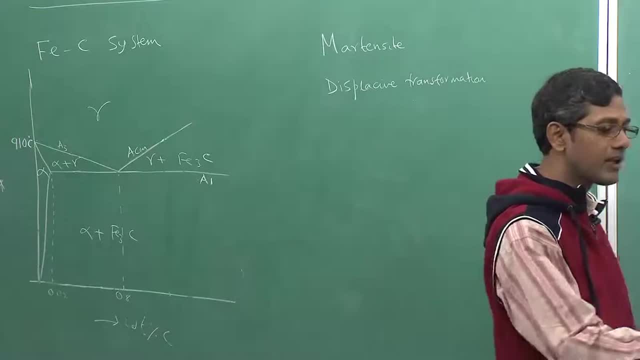 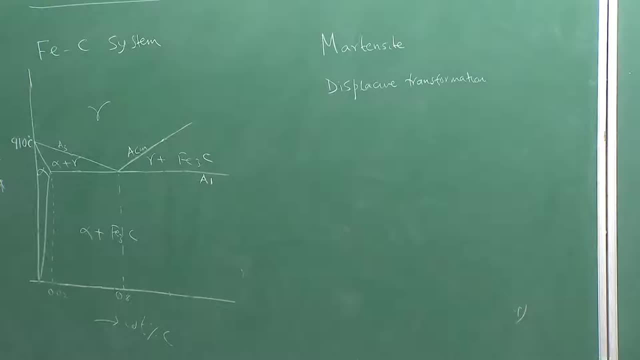 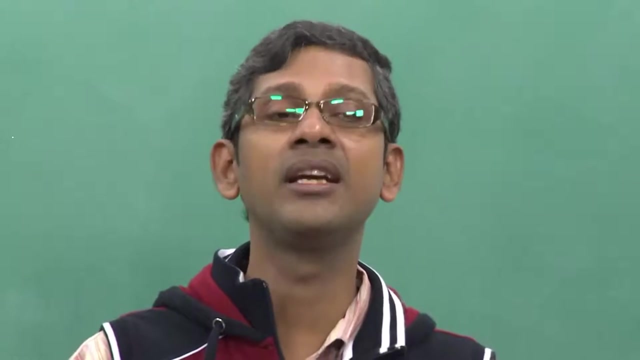 Now question is this: Why this transformation is very important. When Martin discovered these transformations, he did not realize one thing. He thought it is unique to the iron-carbon system. but that is not the case. Martini transformation happens in non-ferrous system. nickel-based hours. 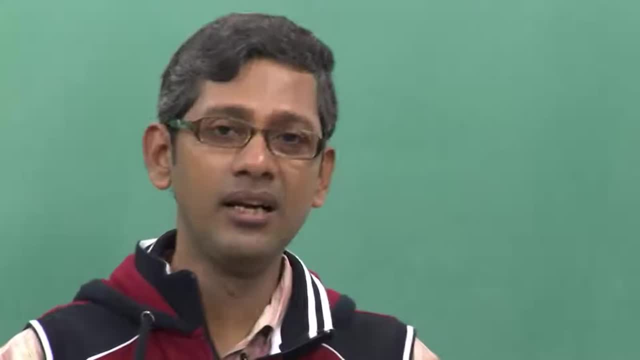 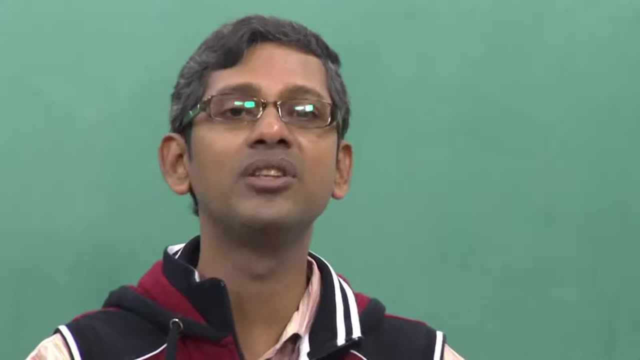 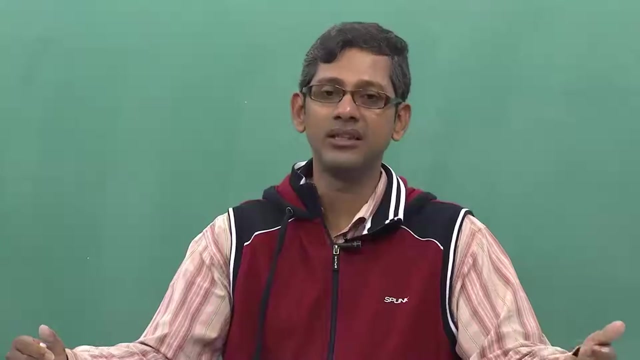 In fact, if you are intelligent enough, the same memory alloys actually depends on this martensite transformation. The same memory effect depends on the martensite transformations, Only thing which will change if you look at martensite transformation in non-ferrous alloys. 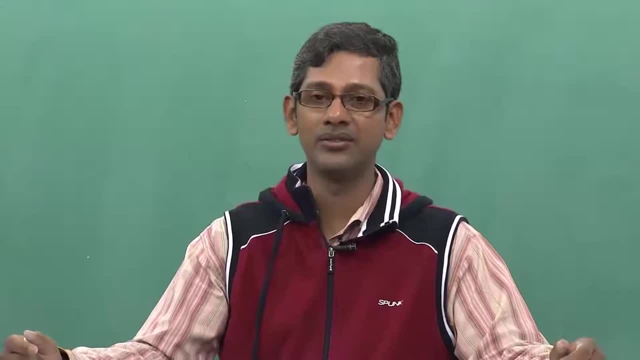 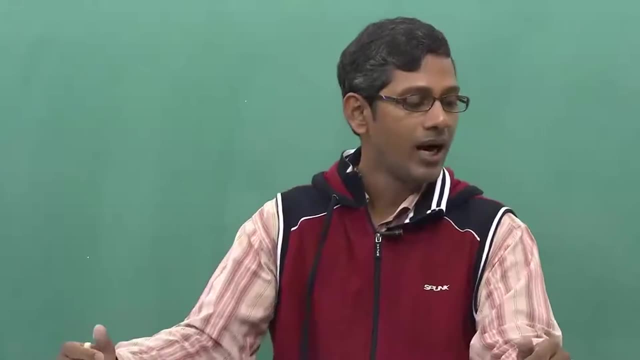 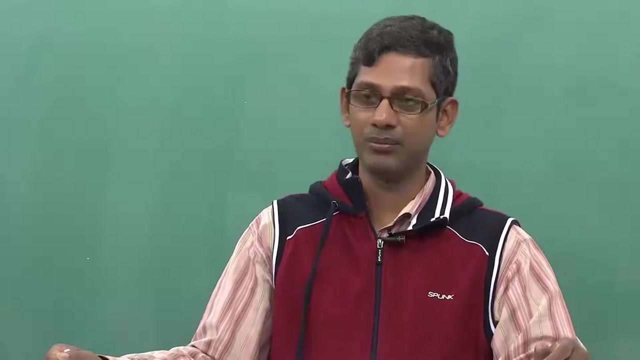 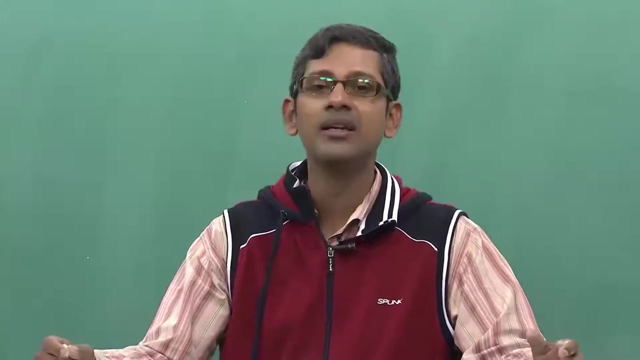 is how the things actually happens in minute details. Otherwise, the mechanism of transformations- a displacive type transformation- will remain same. How does it happen? This happens by cooperative movement of the atoms, cooperative movement of the carbon atoms. The best example, what one gives, or one normally gives in this case, is very simple. 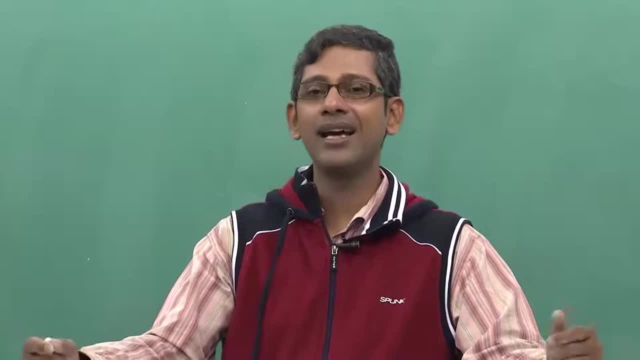 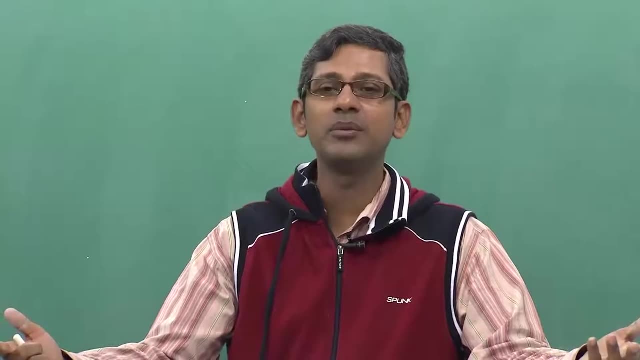 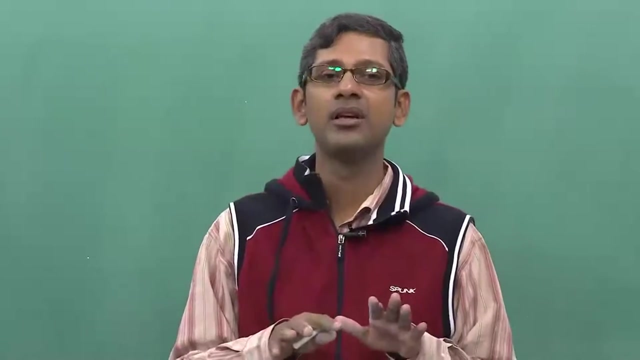 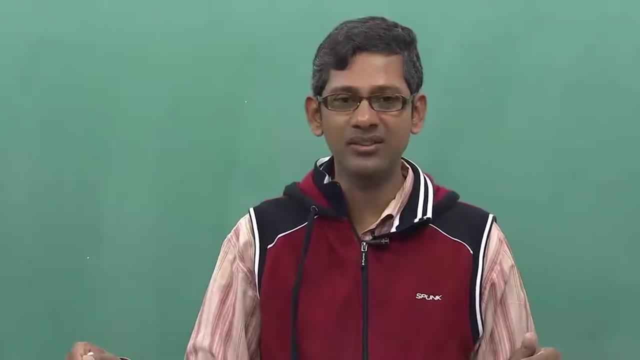 Suppose you are sitting in a classroom and the chairs in the classrooms are actually lattice points, correct? Now, phase transformation means what Structural change, large rearrangement of the atoms? That is what is called phase transformation. If you want to make this change in the way the chairs are arranged in a class, you can. 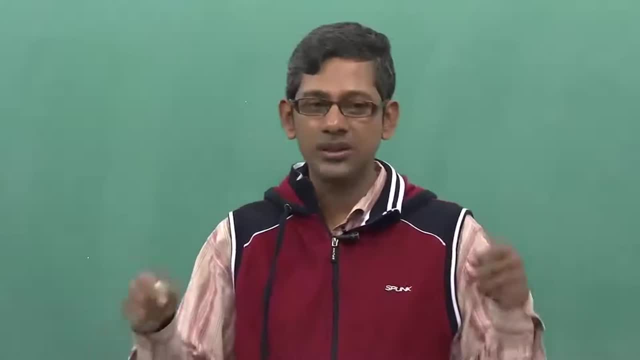 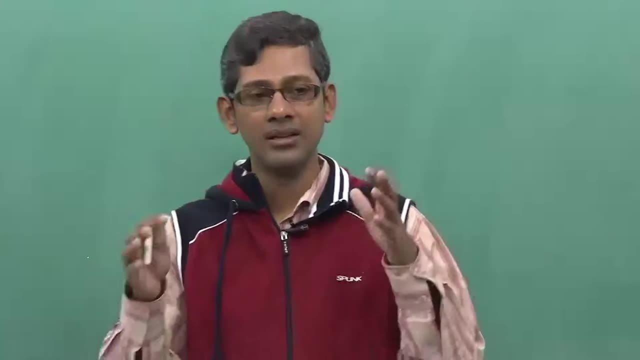 do two ways. I can allow the people sitting in the chair to move from one place to other. That you can do. Then what will happen? The transformation will take place. There will be large change of the atoms on the lattice. Otherwise you can apply force. 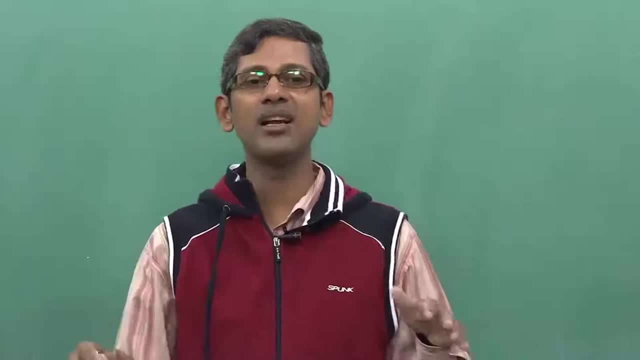 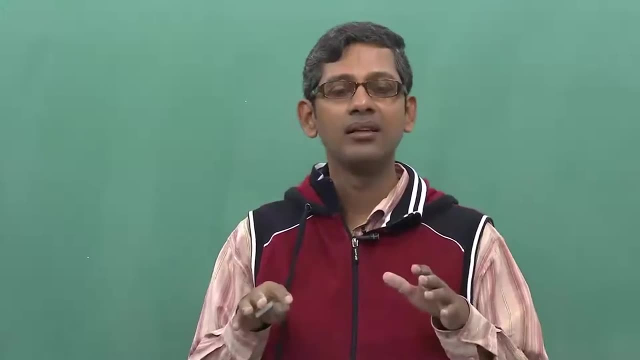 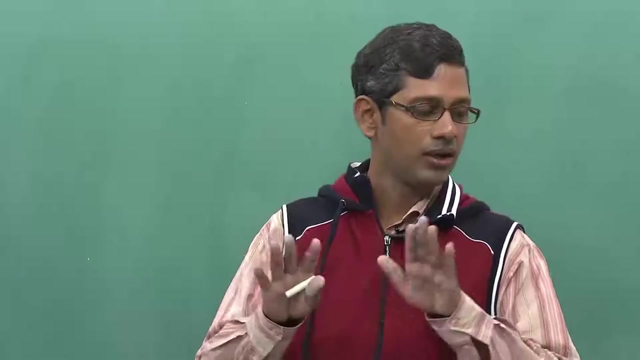 What happens? What happens? You can actually apply force, just like the teacher can use a stick. You can apply force and allow the students to suffer. and that is what happens in modern transformation. In modern transformation, carbon atoms actually move a little bit in the lattice in the directions. 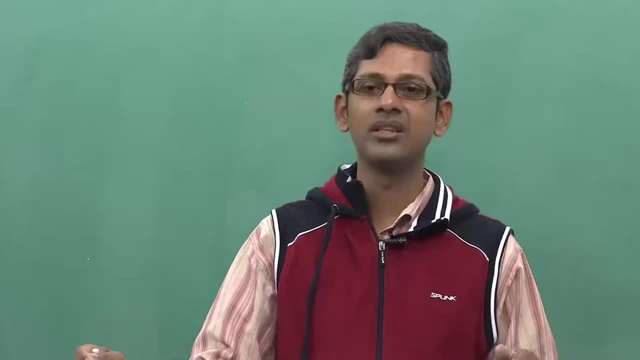 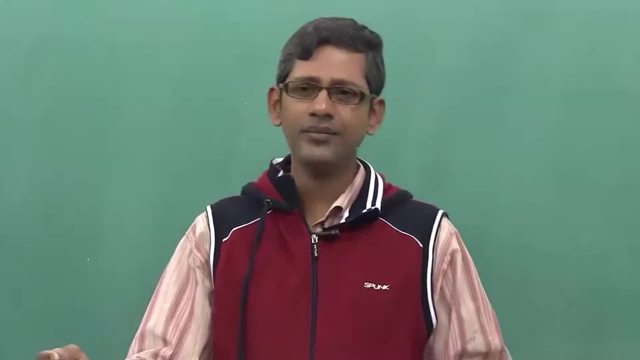 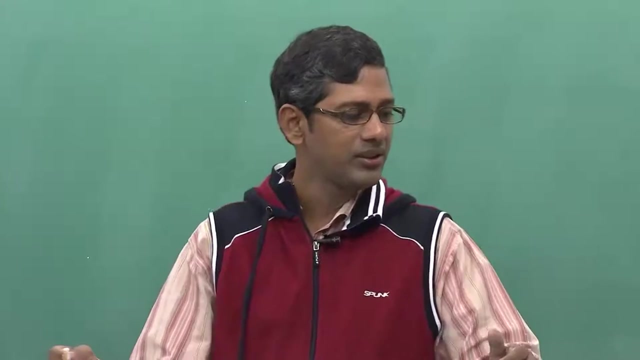 of z, x and y and make this transformation happen. So that is what actually called. that happens because of shearing application, of shear forces. I will not go into exact details of this transformation, but I will tell you few important facts. Deformation happens to accommodate the change in the shell. 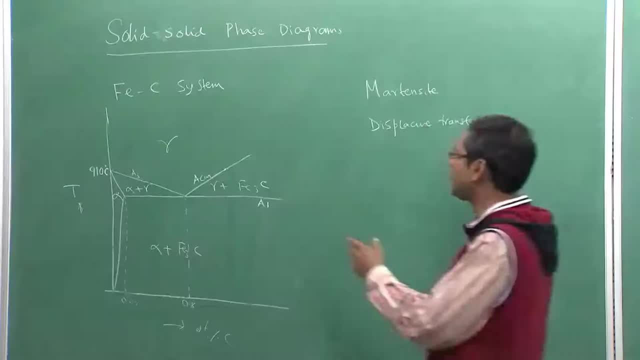 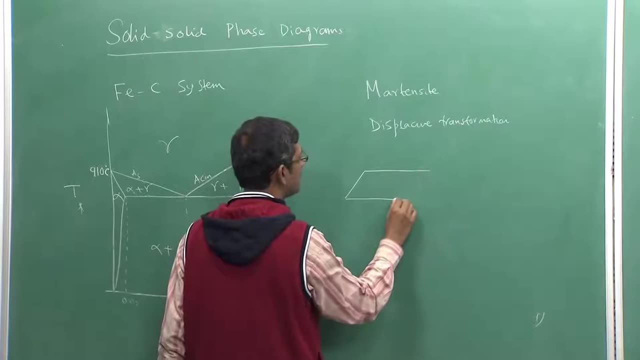 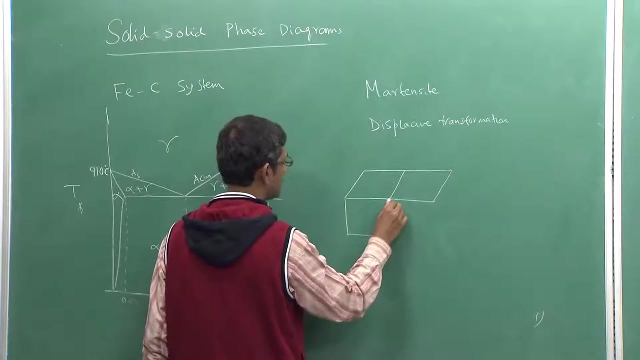 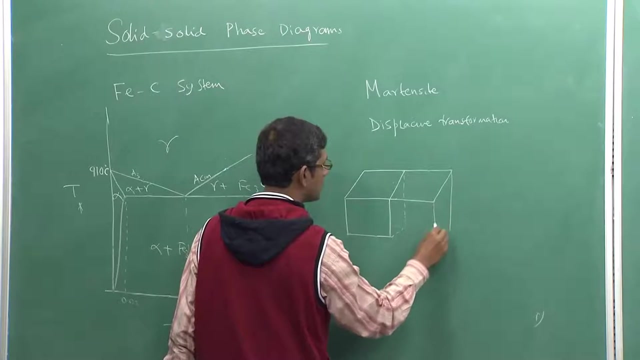 How does it happen? Let us look at it As you know, gamma is basically a FCC phase, So I will draw two FCC in itself and I can show you nicely how this transformation happens side by side. Okay, What happens in this reconstruction if you drink a beer without clicking a button? 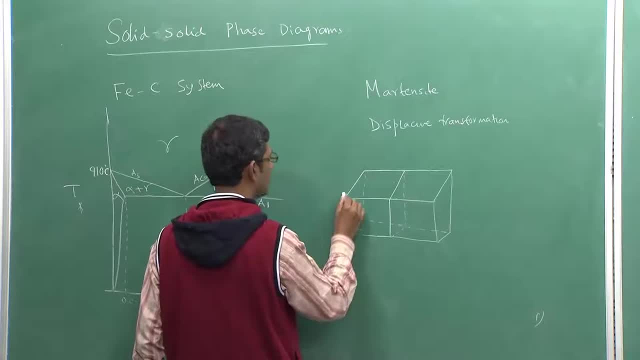 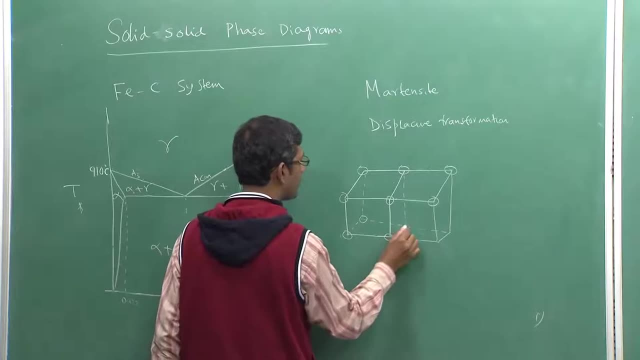 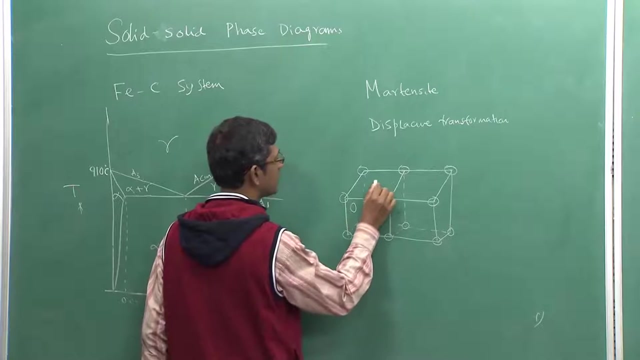 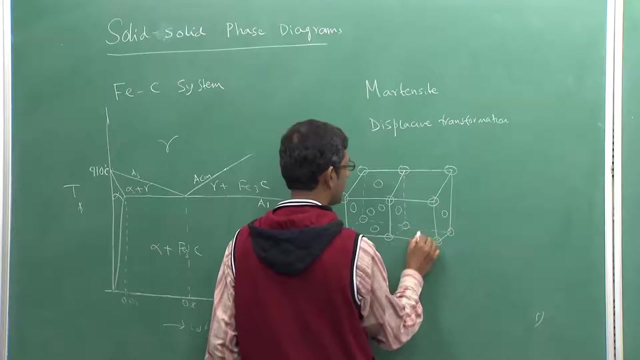 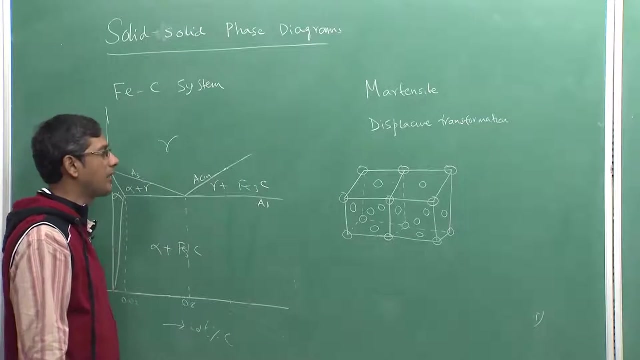 So this is the time frame of this. So the FUCK is called as preload, So it is a just a preload. Okay, What is the下去 coefficient? These are the forerunner phase central iron atoms. So carbon atoms obviously will be sitting in the interstitial phases. 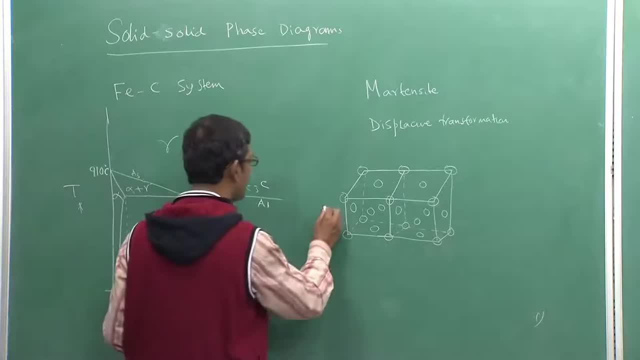 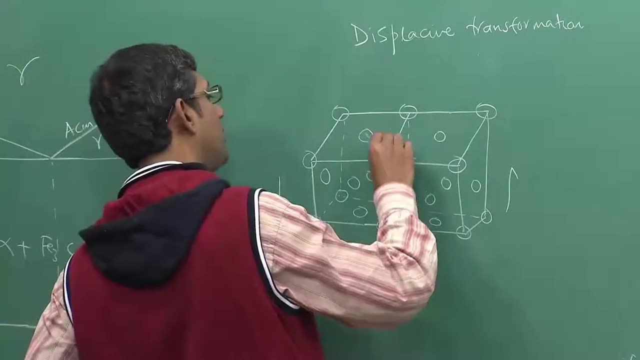 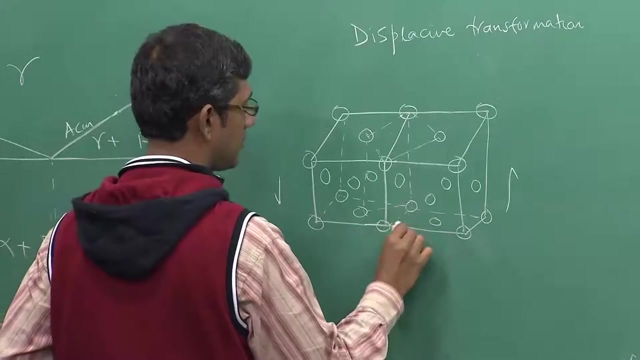 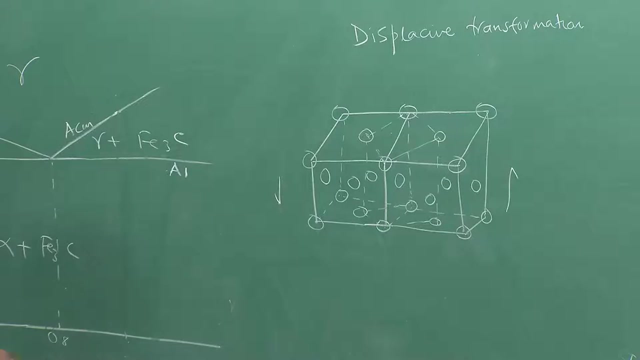 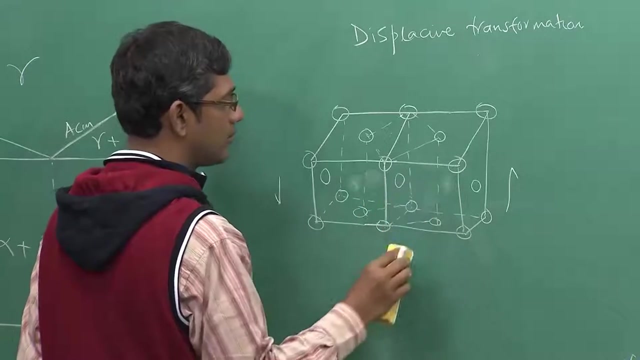 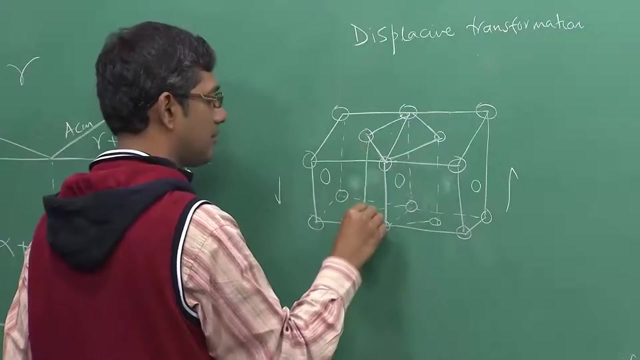 Now I can apply stress, I can apply shear force like this, distort the lattice in such a way I can form this. So let me remove some of the atoms, then you can see it very clearly. so these atoms. So now you can see I have generated a unit cell like this: 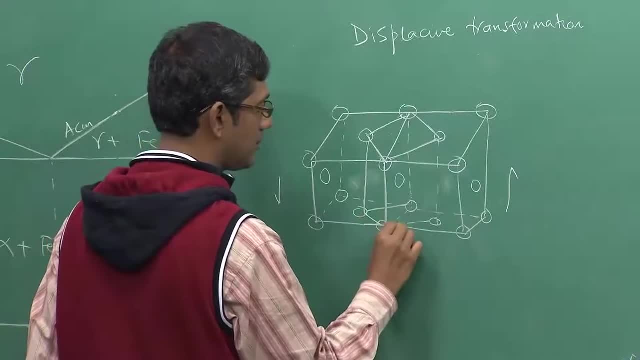 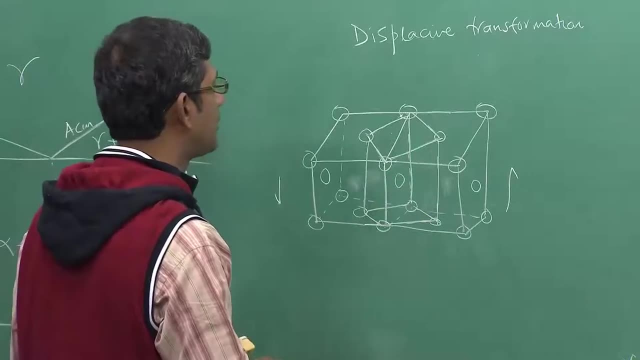 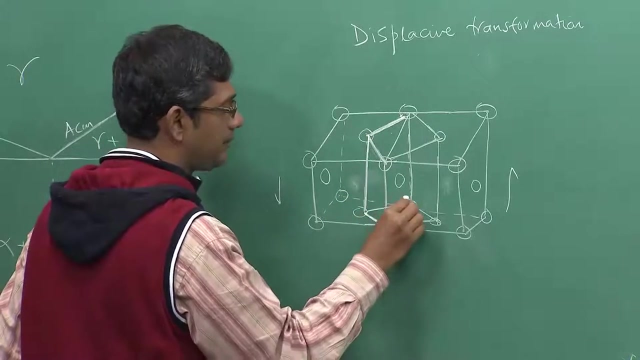 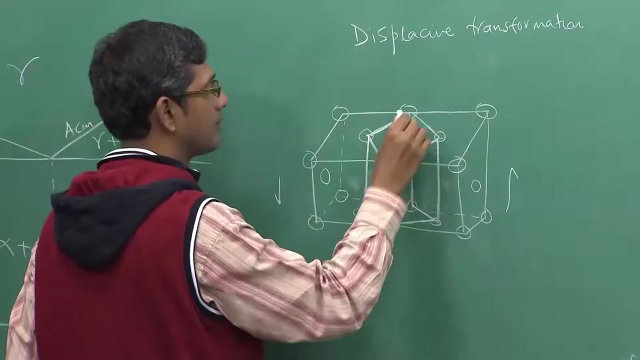 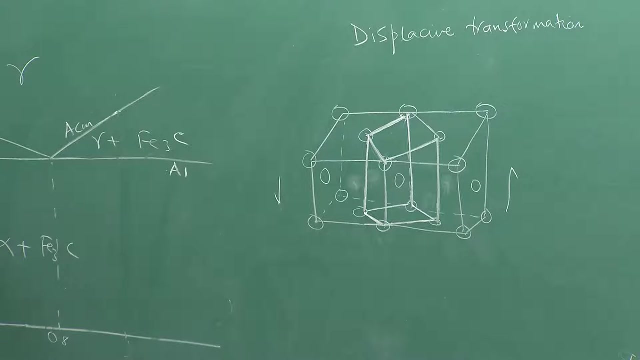 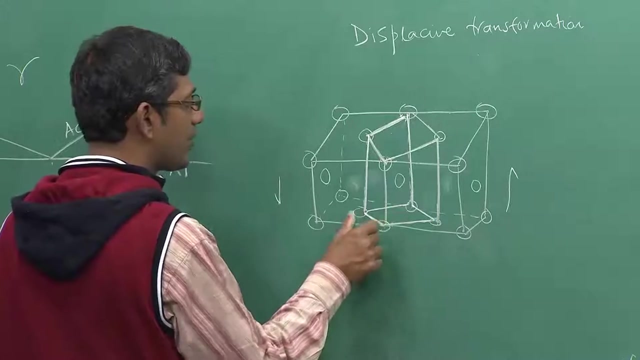 So what I will do is I will make it thicker so that you can see it properly. So you can see, this is the body center, tetrahedron. This is body center, but tetrahedron is because this side and this side, these two sides, have. 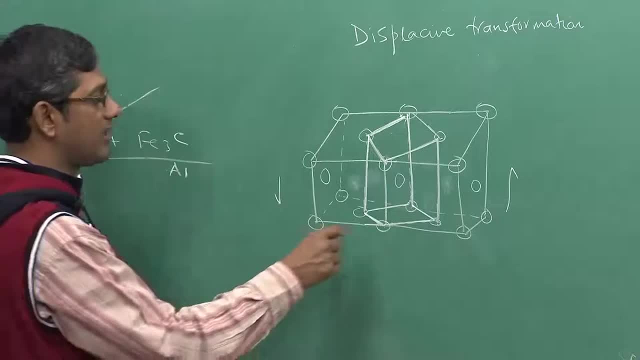 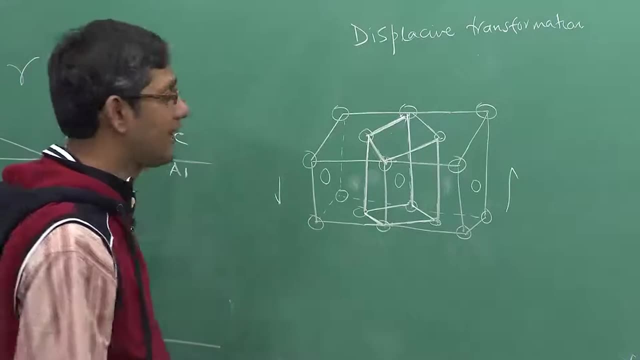 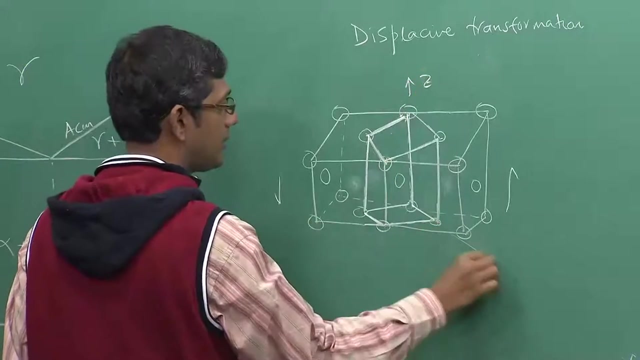 equal length, Although they are looking different length, but they are equal. As you can understand, this is a diagonal, phase diagonal. So phase diagonal should be equal length. but this one is the side of the unit cell. So that is why one of the axis which is suppose, this is Z axis, this is X and this is Y and 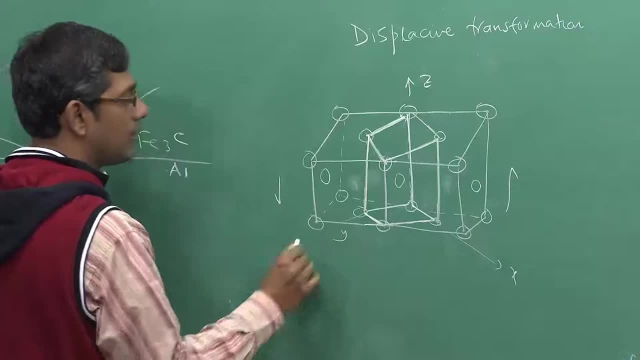 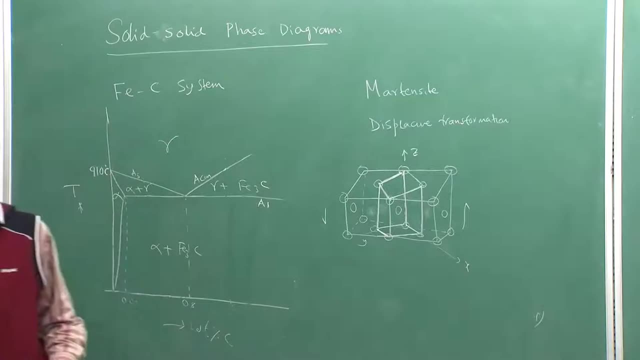 this is Z, So this is Z axis, This is Z axis, So one of the axis is elongated because of this transformations. So what we have done, We have not asked the atoms to diffuse, We have asked the atoms that they are shuffling positions, just like a shuffling of playing. 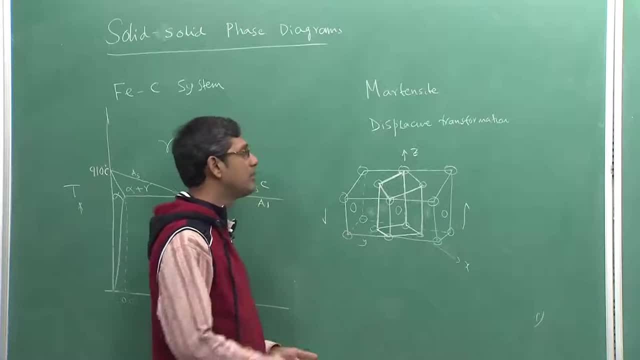 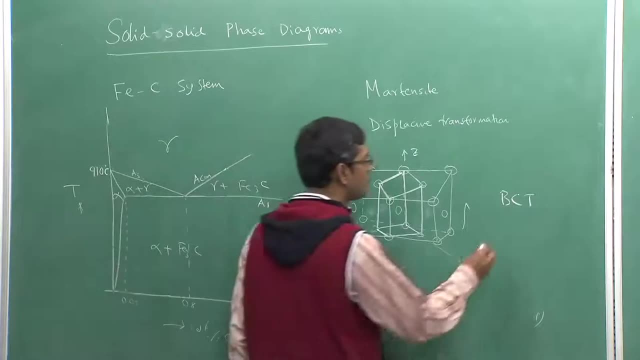 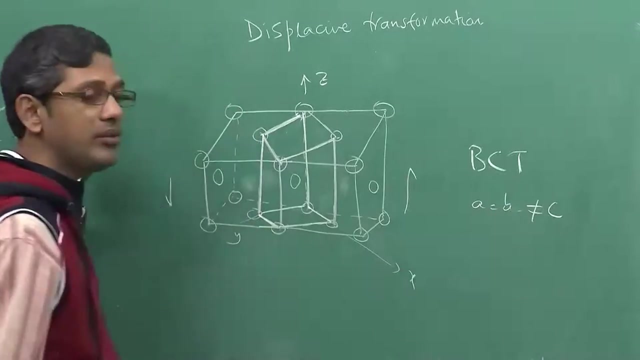 cards. So by doing that you create a unit cell which has a body center, tetragonal structure, and this tetragonality is very small. In a tetragonal unit cell, A is equal to A but not equal to C, Correct, Or A is equal to B rather not equal to C. 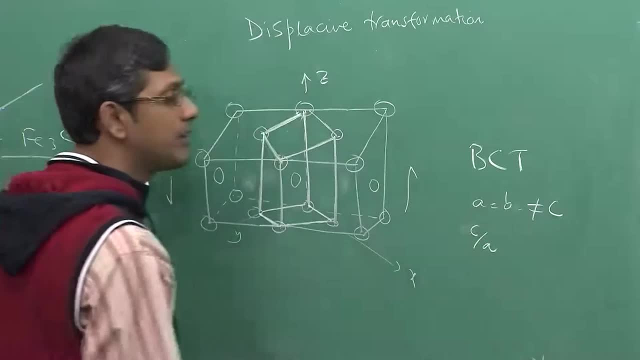 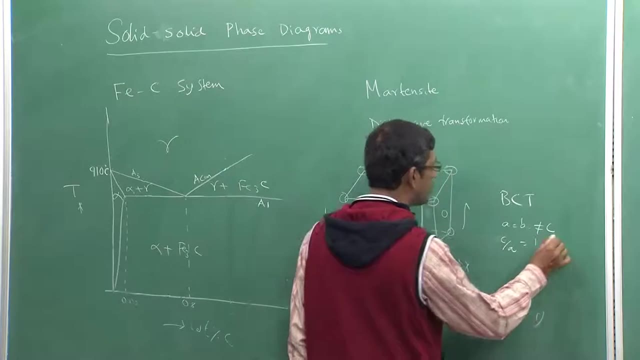 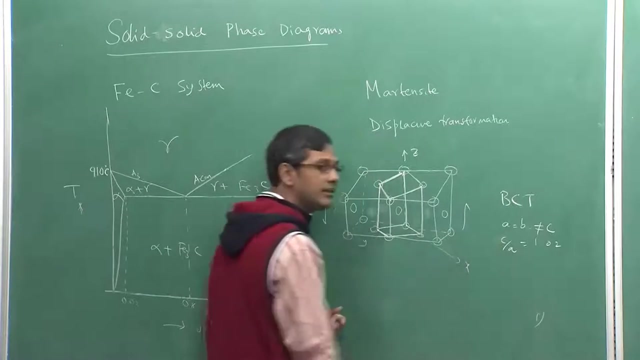 So therefore, most important factor in a tetragonal cell is the C by A ratio, which tells you the tetragonality of the cell. Here it is very small. This may be 1.02 or something Very small. So there is a small difference, very small difference in the C length of the C axis. 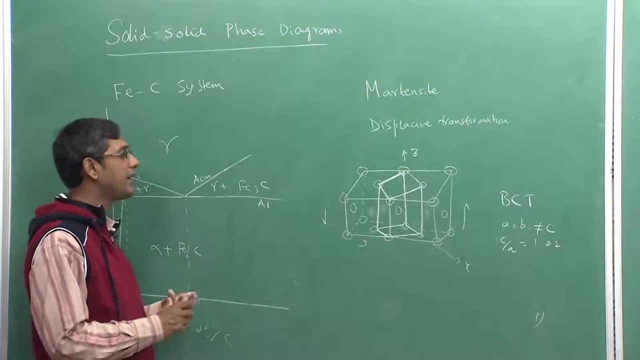 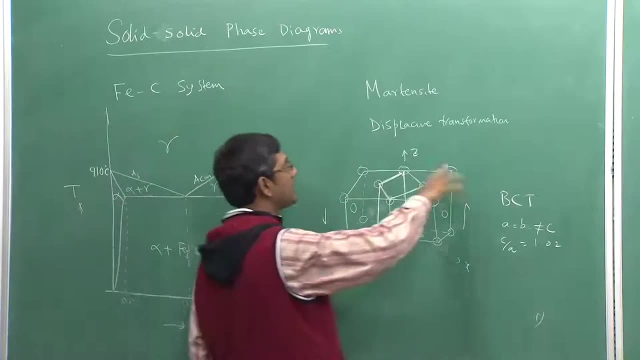 as compared to A axis. but this is the way the transformation happens. Now question is this: So that means what? We are distorting the unit cells and this happens in like this: You have a line number of FCC unit cell sitting like this: 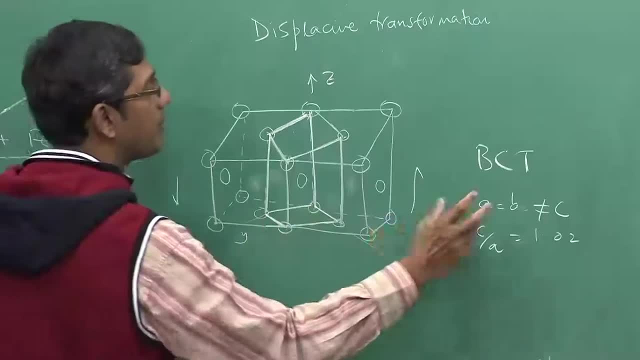 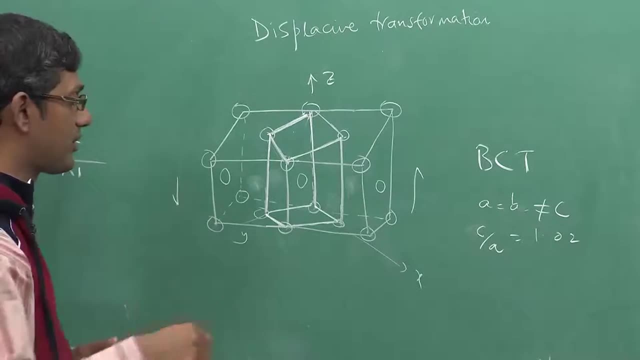 So this happens by flipping. You, flip, flip, flip. So all the unit cell will get changed and this can happen with speed of sound. That is why martensite transfer is so fast. You take the sample at 950 Celsius temperature. it can change in water. 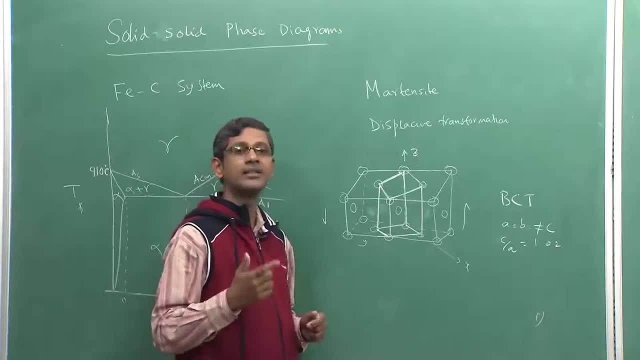 Immediately the steel gamma will transform to martensite. That means the rate of transfer will change. That is why martensite transfer is so fast. The rate of transformation is just like a speed of sound inside the steel. That is very high. 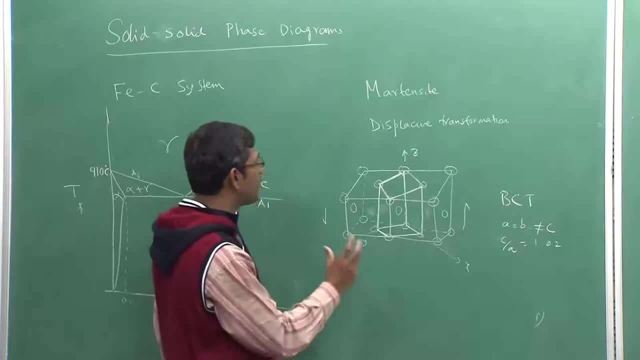 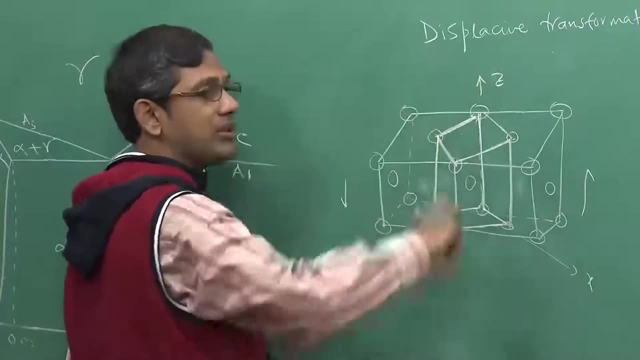 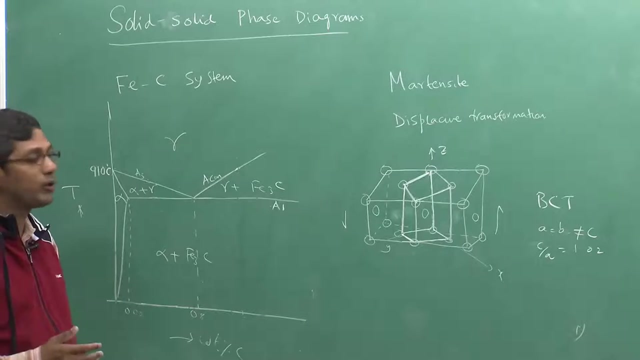 Speed of sound is very high. Now why this happens? speed of sound? Because what you need, You need basically to flip the unit cells, just like that, from this position to this position. That is easy to understand, Everybody can understand this. That is what actually leads to deformation of different domains. 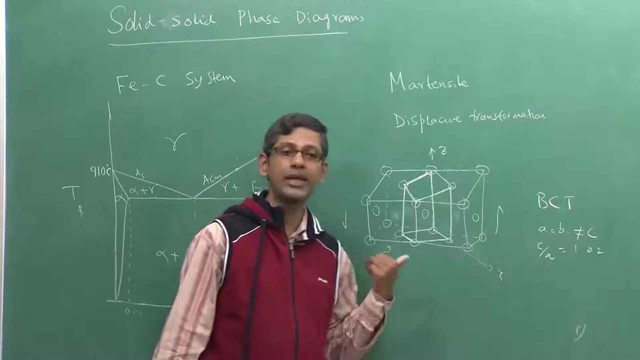 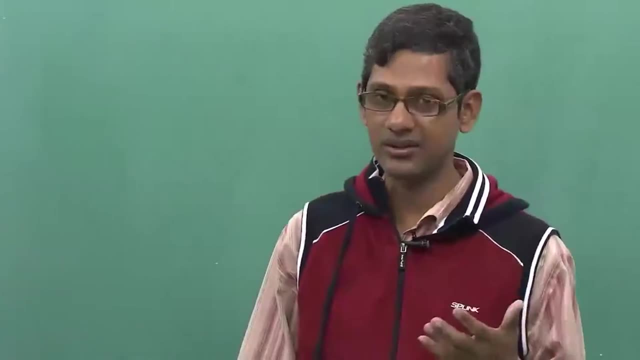 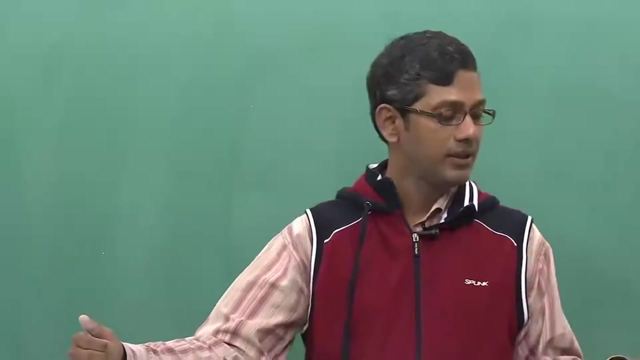 But if you look at carefully, there are two types of deformation happens in such transformations: One which will lead to change of set or change of crystal structure. rather One which is leading Change of crystal structure means from FCC to VCT. the way I have shown is y by 1.. 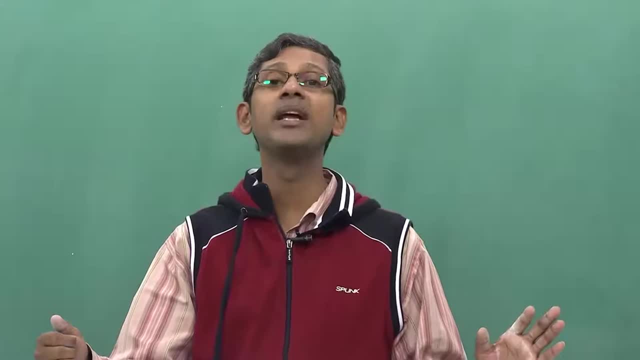 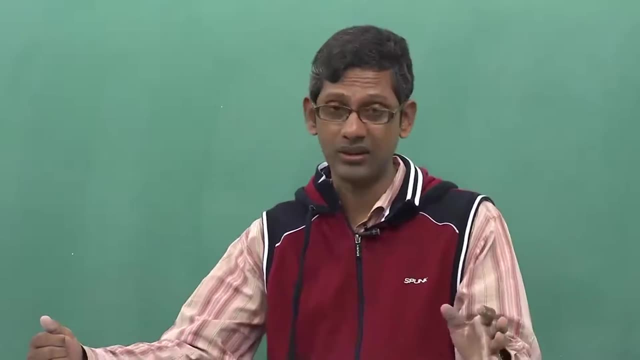 This transformation is known as homogeneous plane strain change. This transformation is done by homogeneous plane strain. Plane strain, you understand The strain in which one of the component- third component- is not present. That is why it is called homogeneous plane strain. That is why it is called homogeneous plane strain. 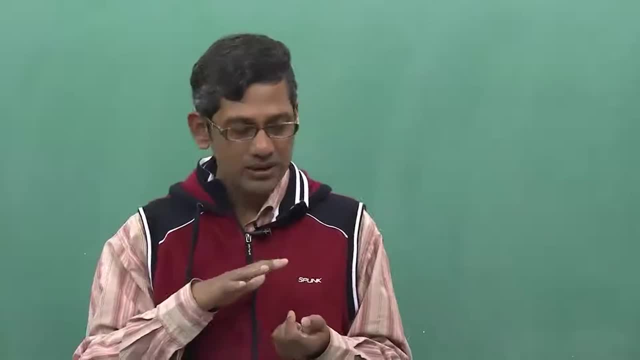 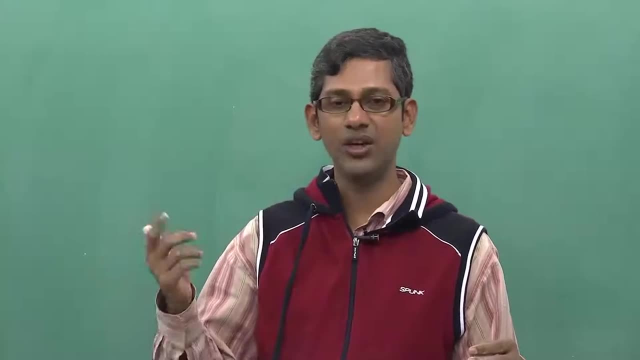 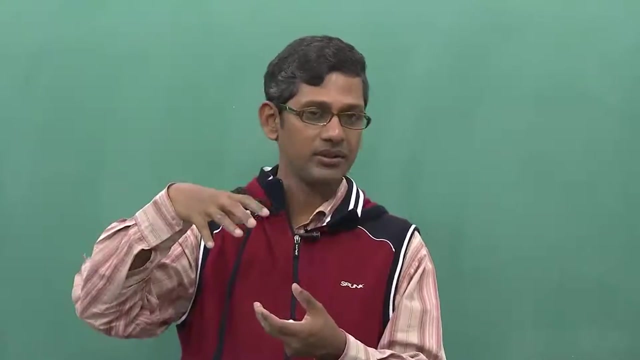 That is why it is called homogeneous plane strain, That is why it is called plane strain situation. So that means you have a plane strain situation in which the crystal structures get changed from FCC to VCC or VCT. So, and in this case, what happens for the plane carbon steels? there is a 20% compression. 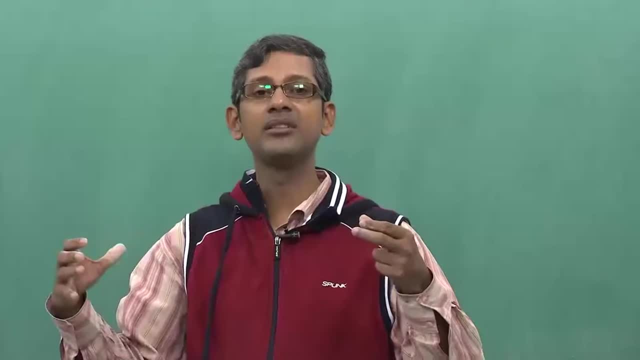 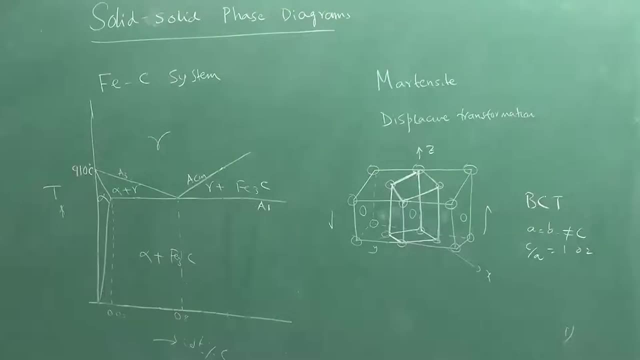 along the C axis and 20% tensile stress or tensile strain along the X and Y axis. So along the Z axis there are 20% compression. It will be compressed. On the other hand, along the X and Y axis there are 20% compressions. 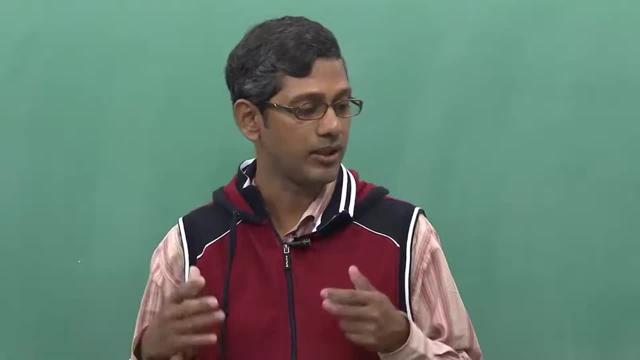 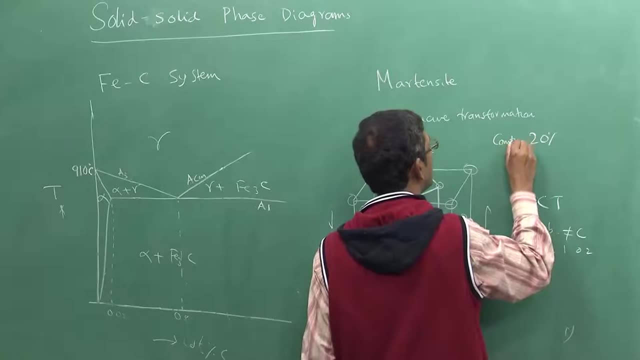 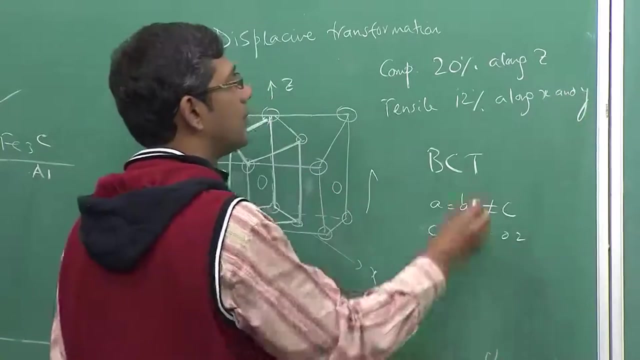 It will be compressed. On the other hand, along the X and Y axis there is 20% tensile, sorry, 12%. let me write down: So along, 20% is the compression stress along Z, but tensile stress of 12% along X and Y. 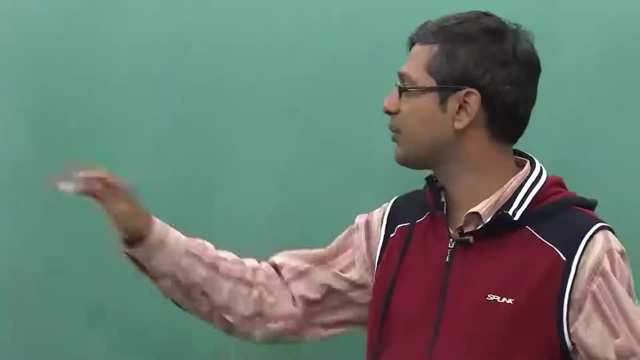 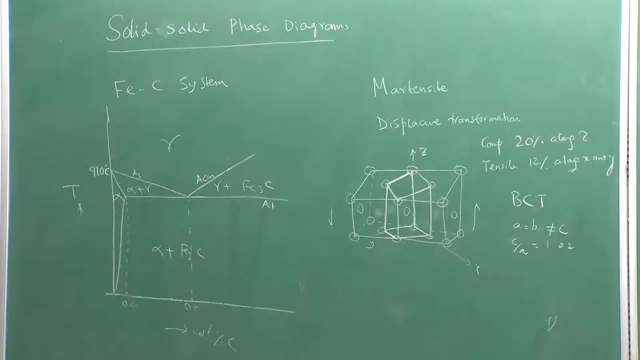 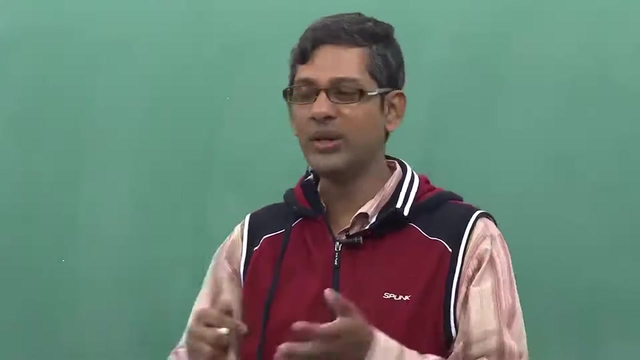 This is the amount of strain applied and this strain leads to change of crystal structure. Just by flipping atoms you can change this crystal structure. Correct So but people who have investigated a lot this martensitic transformation in steel, they have found, although we are changing the crystal structure by applying strain or by 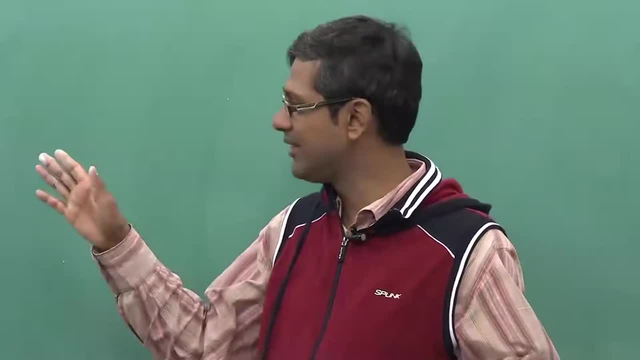 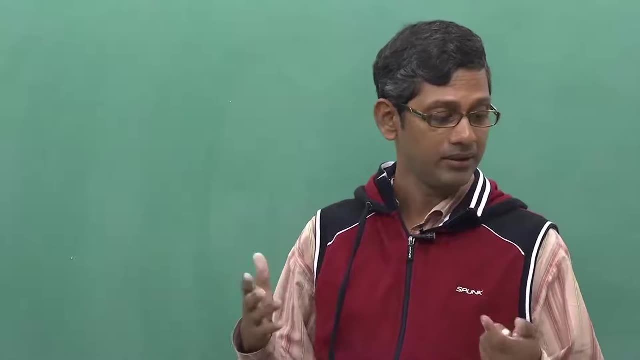 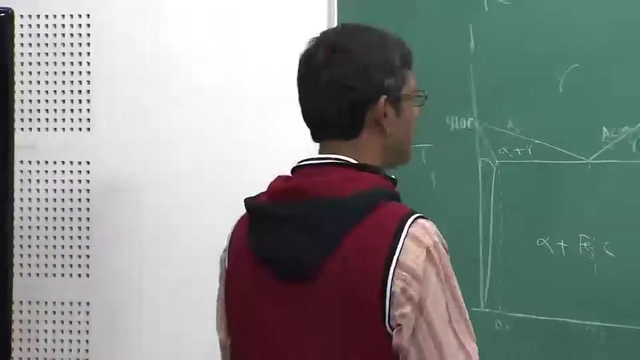 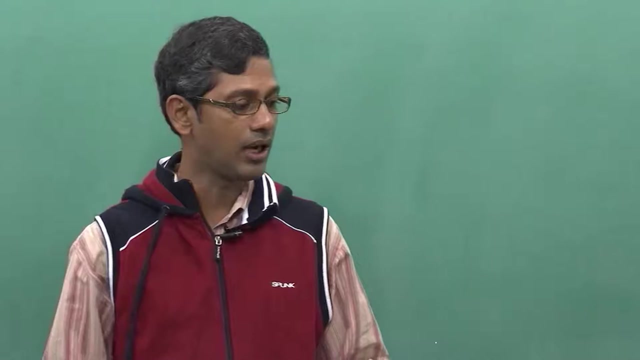 because of shear force, there is a plane in this whole structure which will remain unrotated or undistorted even after transformations. Okay, So this unrotated or this unrotated or unchanged or undistorted structure, known as habit plane, 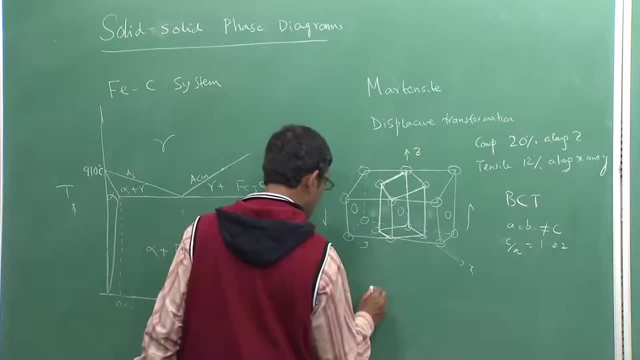 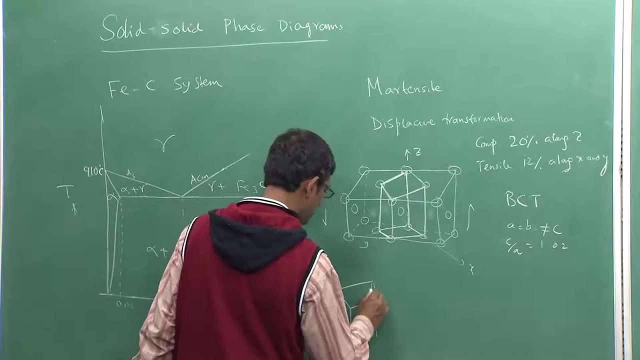 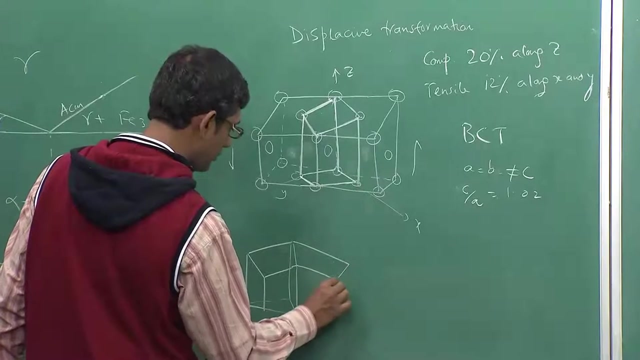 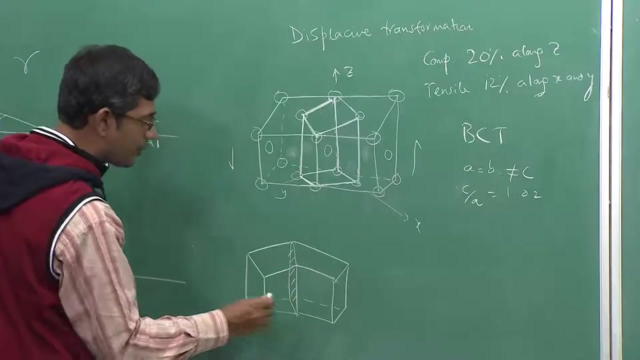 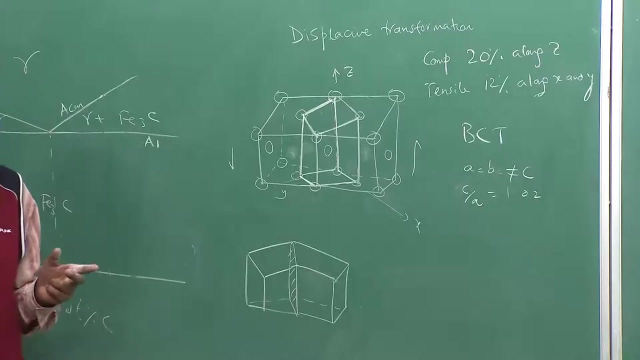 So let me just draw it in a nice way. It is very difficult to do. Okay, Let me get my meshes. So this plane here. as you see here, these two unit cells have rotated. they rotated this way, but this one has not undergone any rotation transformations, any distortion. 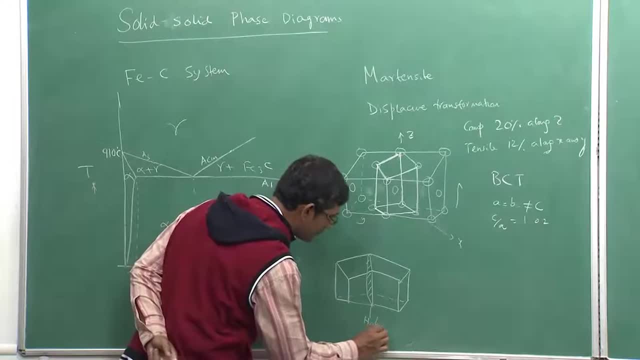 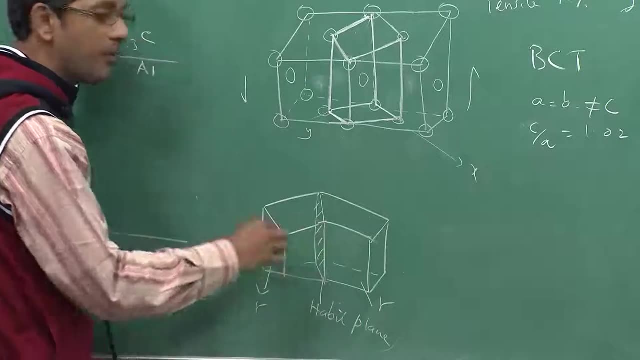 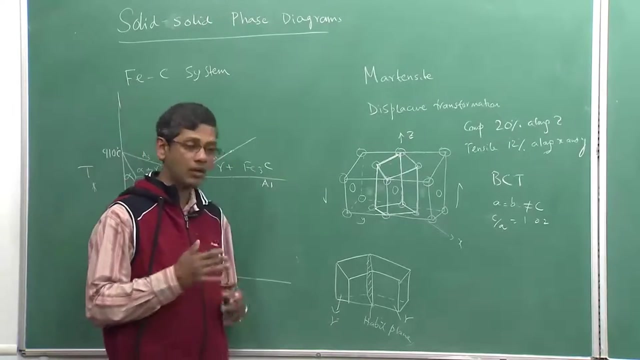 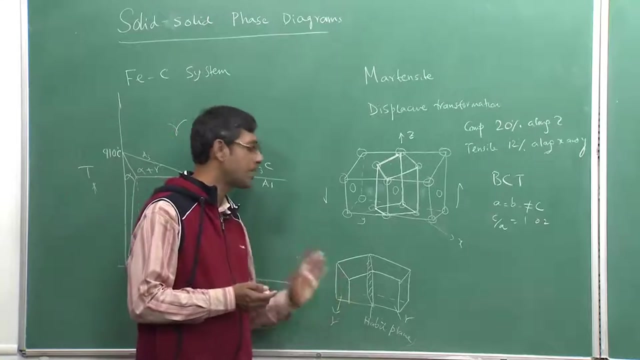 So this is known as habit plane. This is gamma. this is also gamma. this is the martensite. So in the martensite, one of the plane will remain undistorted, or no change of the shape or whatever positions. that is what is known as habit plane. 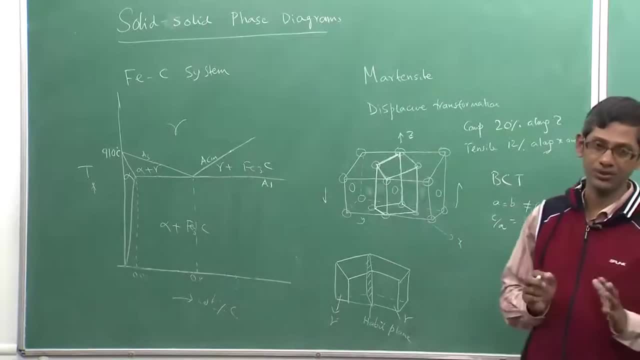 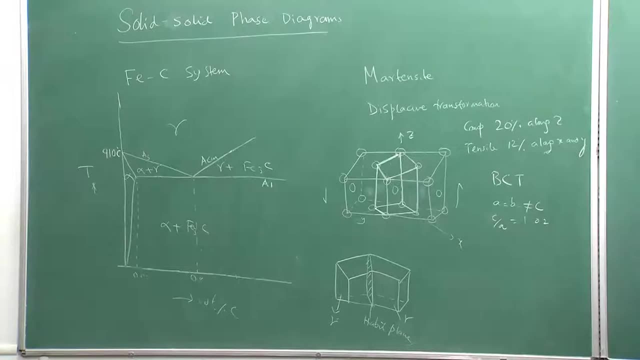 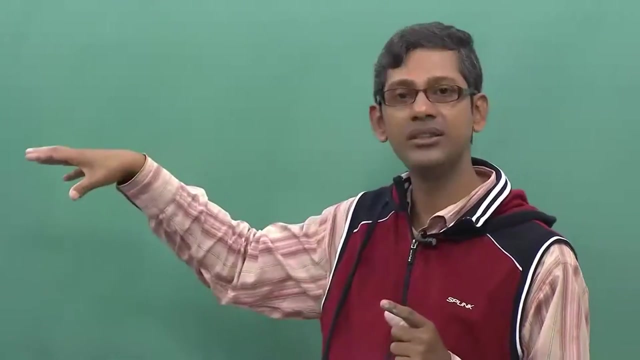 So this plane does not undergo any kind of distortions. So thus, in order to keep this plane undistorted, you need certain deformation to happen, because you are already deforming the whole crystal. you are changing the shape of the crystal. you are changing the shape of the crystal from FCC to BCT. 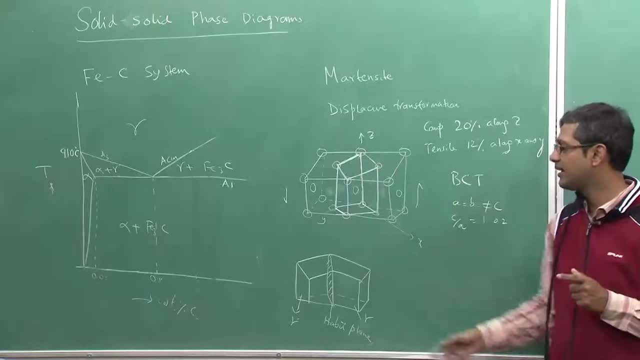 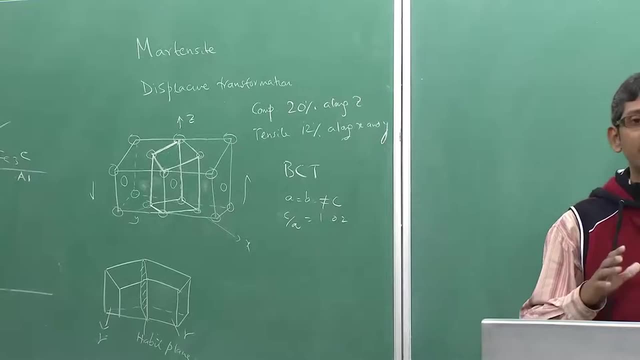 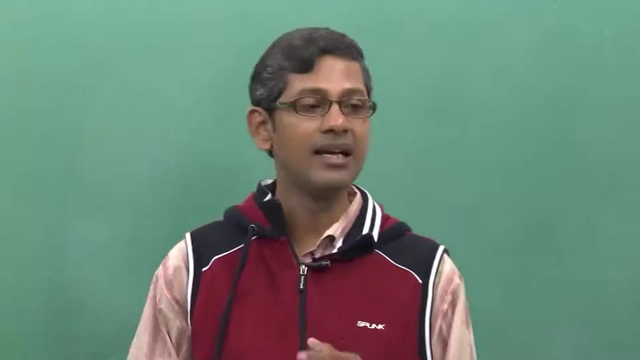 And within this martensite, one of the plane is remained undistorted. How it is possible? That is only possible when you are having somewhere else. the strain is applied to accommodate the strain because of the effect of this plane, and that can be done either by slip or by. 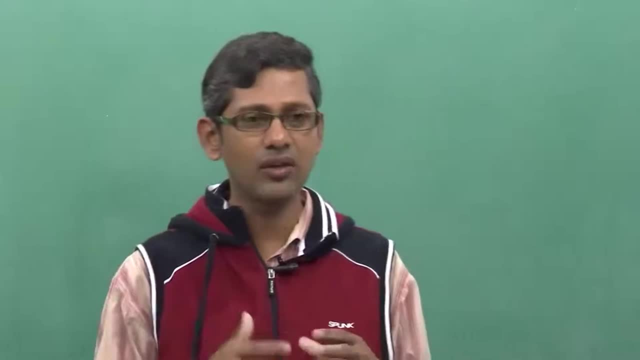 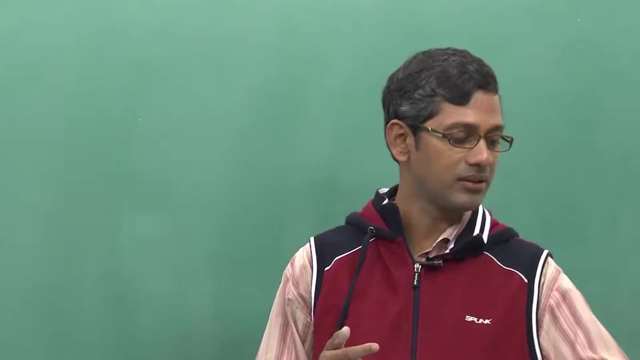 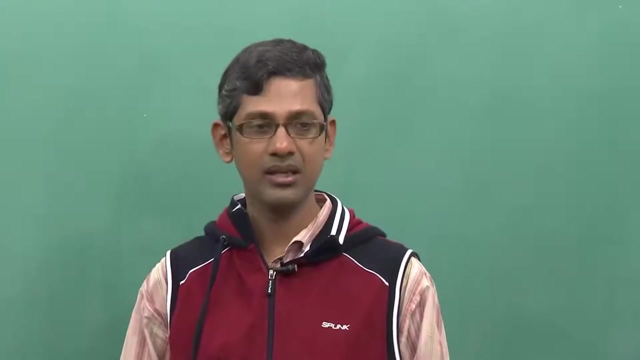 twinning, Although it is very difficult for you to understand or for you to visualize, but that actually happens in the real steel, and that is what is known as. to keep this unrotated crystals in the same position, we need to apply either slip or twinning. 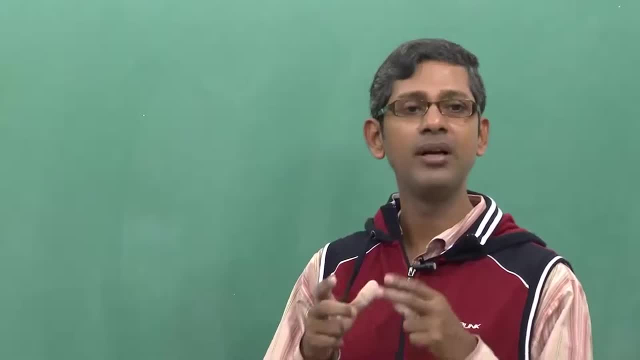 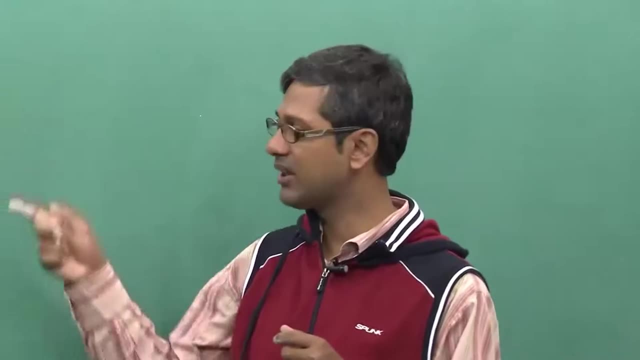 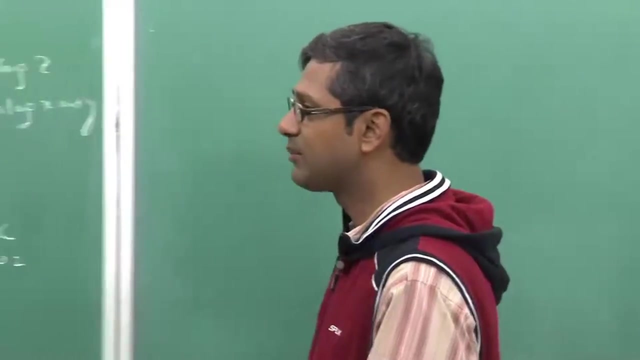 That is why you see- I will show pictures also. that is why you will see lot of deformation twins in the martensitic plates, and this deformation twin is to accommodate the strain which is required. How to keep this plane undistorted? Well, few important aspects before I finish this lecture. we are going to discuss more. 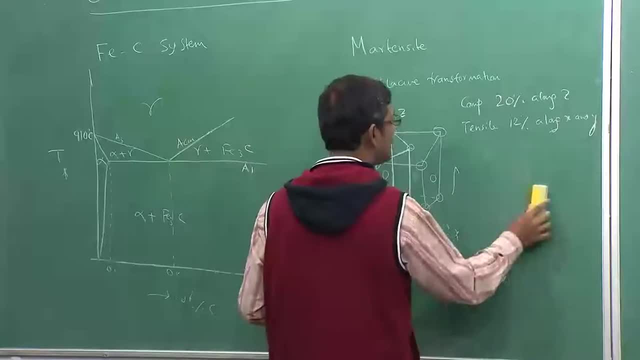 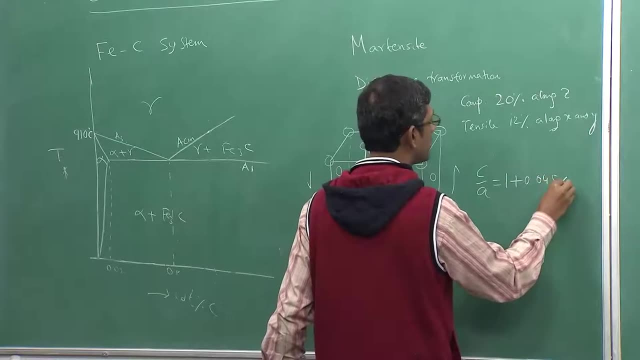 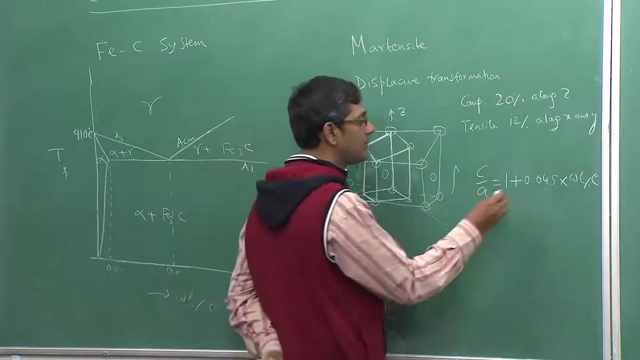 on martensite in the next lecture. also, One is that the C by A ratio, which I told you is basically depends on carbon percentage in the steel. This is how it is, So C by A is basically 1 plus 0.05 into 8% of carbon strain. 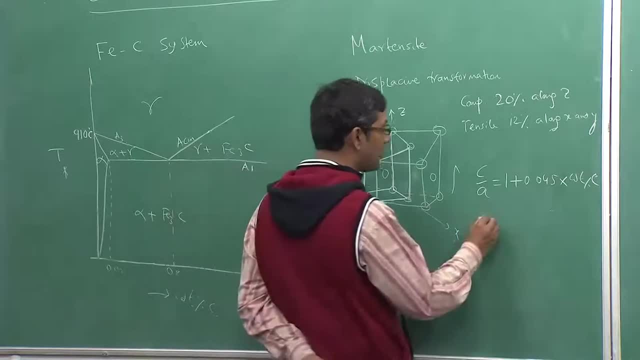 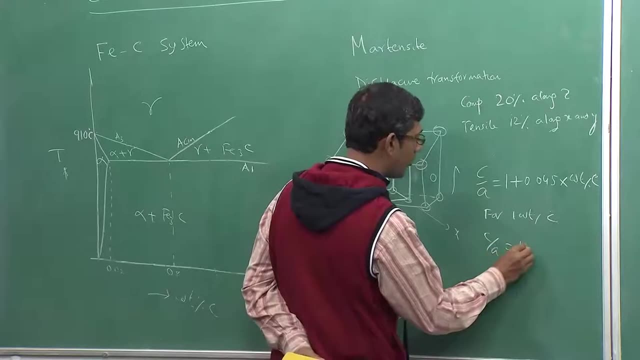 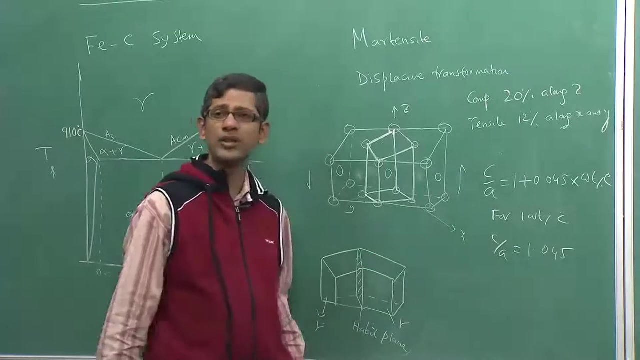 For one weight percent carbon steel, the C by A is 1.045, that is what. This is very small difference between C by A, So your carbon concentration is very low. Suppose carbon concentration is 0.01 percentage or 0.05 percentage. let us calculate it 0.01. 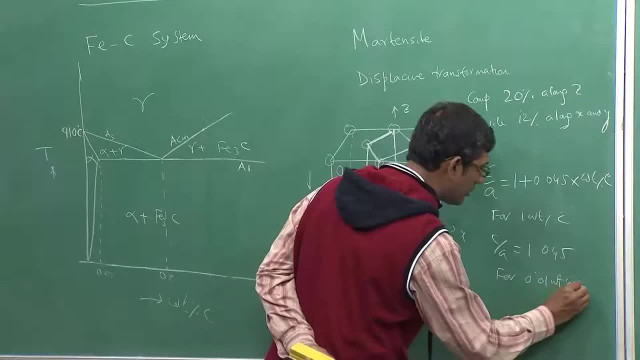 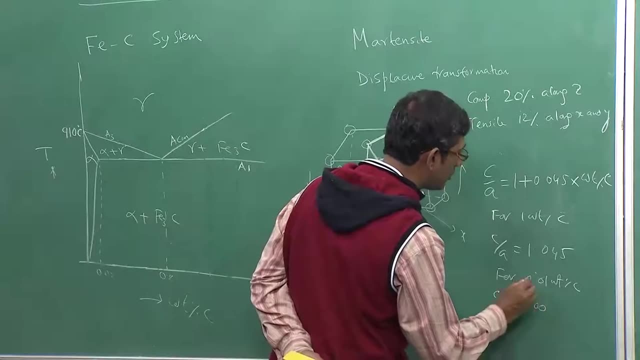 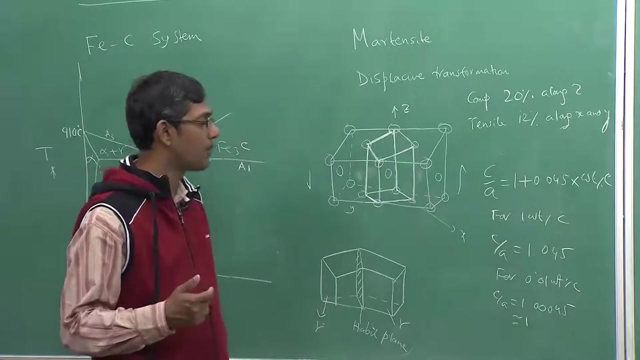 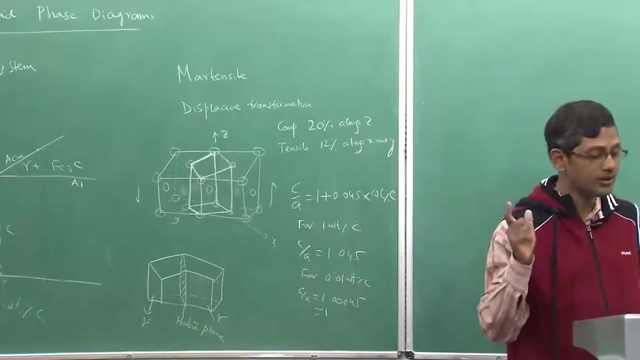 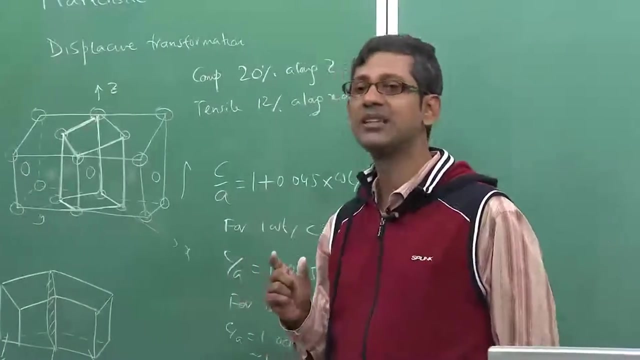 percentage of carbon. This will be C by A is basically 1.05.. 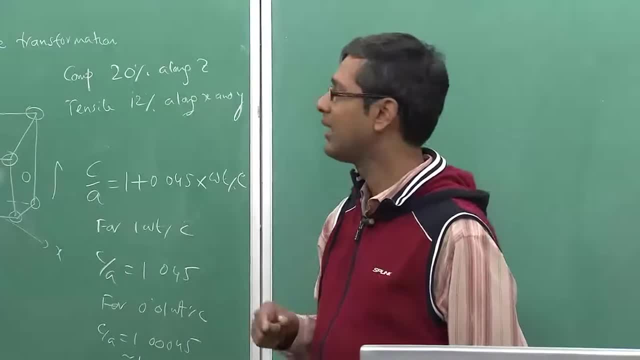 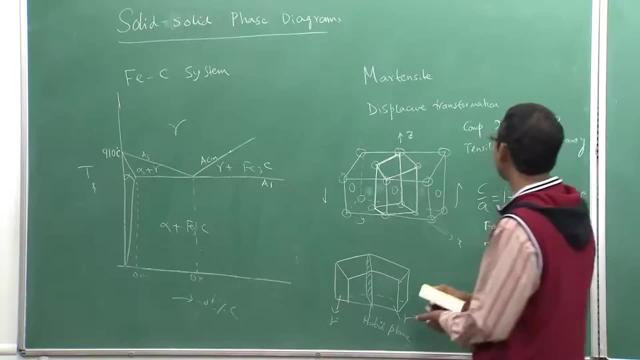 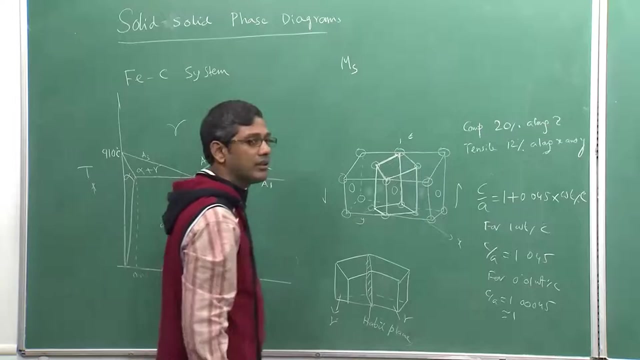 For a particular steel it cannot start in any temperature. Like for pearlite, the transformation starts any temperature below a 1.. For martensite it starts with a temperature is known as M s temperature. always This is what is called martensitic start temperature. That depends on the carbon-caustic steel and it ends with the temperature known as M f. So therefore, this temperature range in which the martensite transformation happens in steel and this temperature is only very low For plain carbon steel, M s is about 200 degrees Celsius temperature. 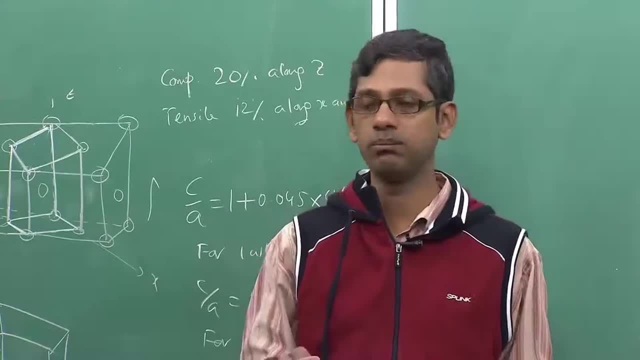 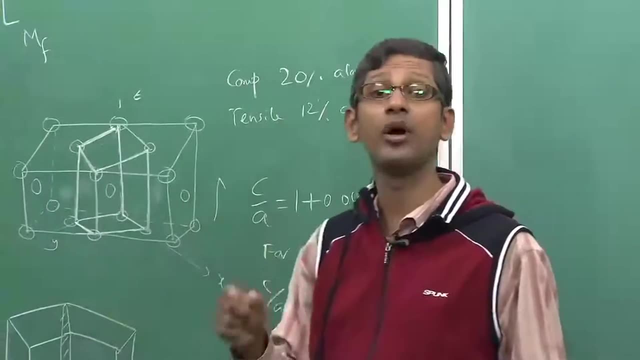 And if you add alloying element this can go up a little bit. So in the next class I will give you the formula of M s temperature, which will depend on compositions of the different alloying elements in the steel. So that is one thing. 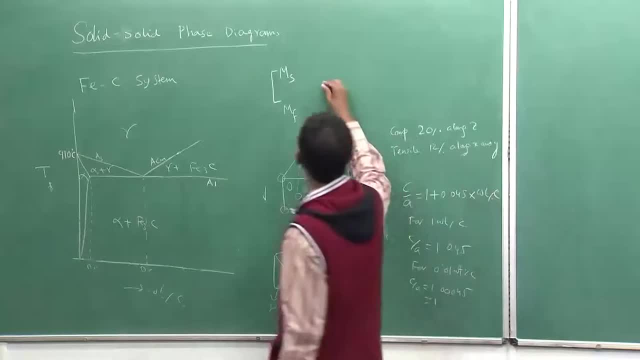 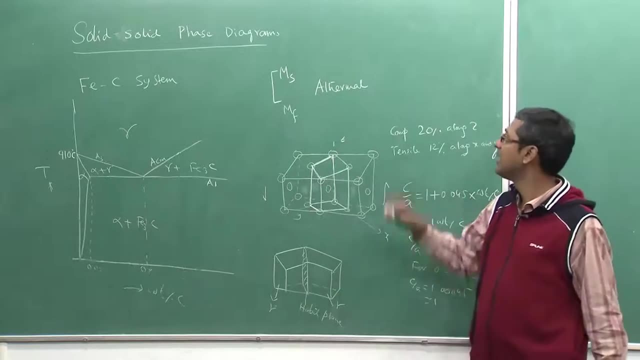 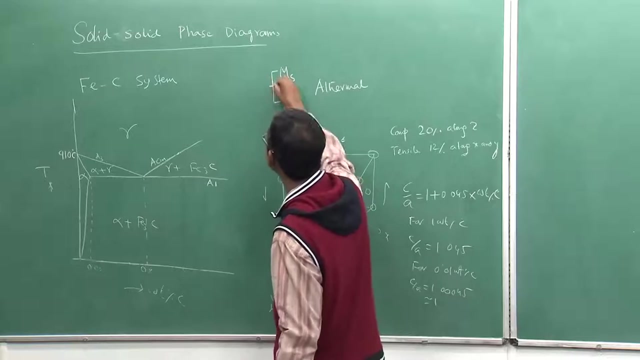 Second important thing: this transformation is athermal in nature. It is known as athermal- These are the terms you will use, You will listen- in steel metallurgy. This is athermal in nature. What does that mean? That means if I cool the sample below M s suppose if I cool it somewhere there below. 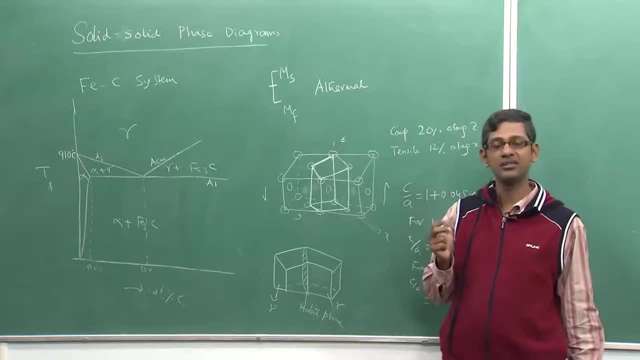 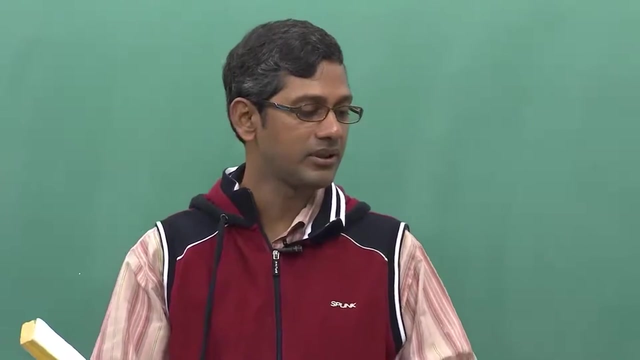 M s transformation will happen spontaneously, as usual, but it will not depend on any further decrease as a cooling rate or something That is what is known as athermal, or rather, I can tell you very nice way: this transformation is basically independent of time. 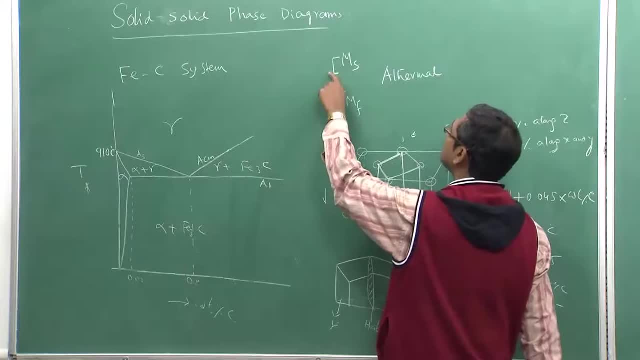 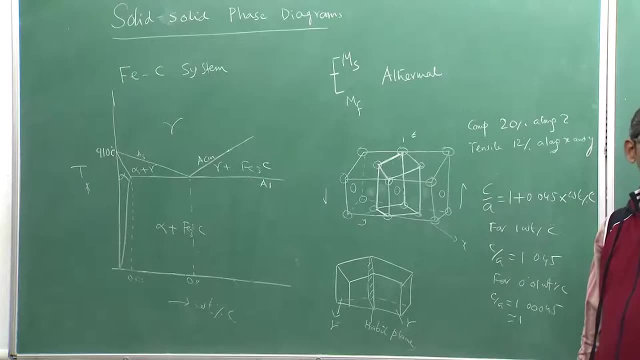 So if I cool it down, the steel below this M s temperature somewhere, here transformation will depend independent of time. It is not dependent on time, unlike pearlite transformation. Pearlite transformation depends on time. there is a rate. So here it depends on the temperature below M s. 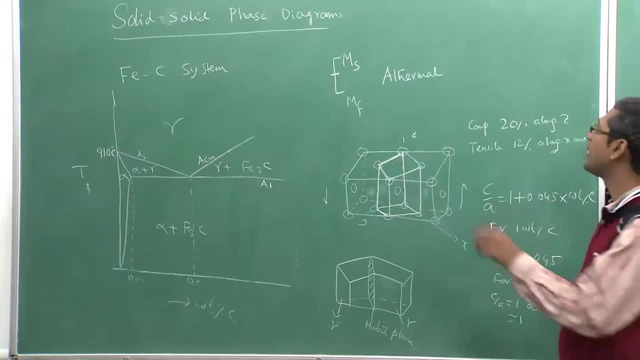 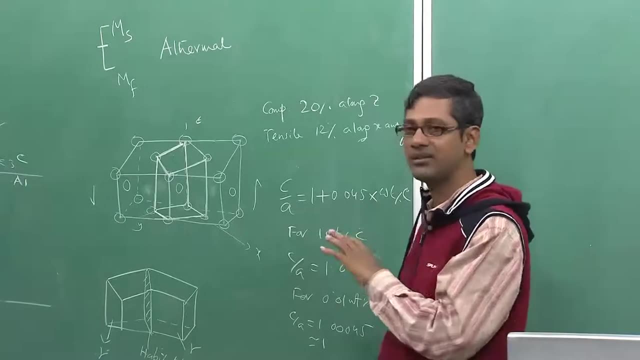 That is all. If you cool it down below M s, it will transform. If you cool it down below M f, it should basically transform fully into martensite. All the gamma grains will transform into martensite, but that does not normally happen. 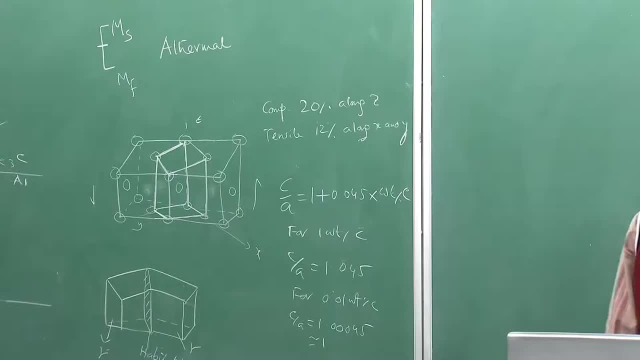 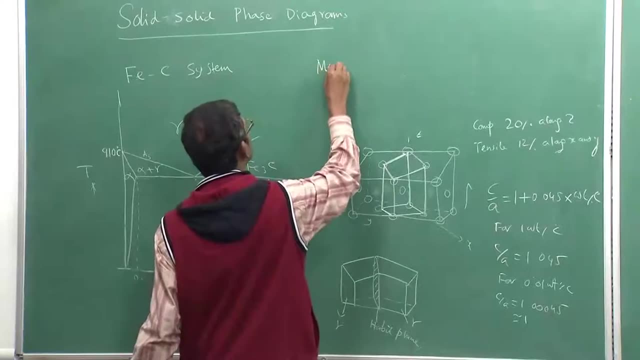 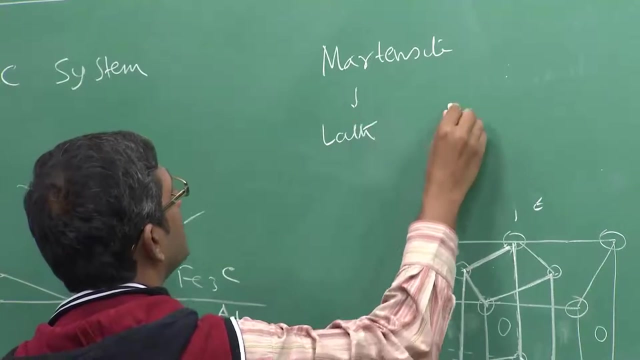 That is one thing you should remember. We will discuss more on this. Last thing which I would like to tell you is that this martensite transformation. martensite have two morphology: One is lat, other one is plate. There are two morphology of martensite. 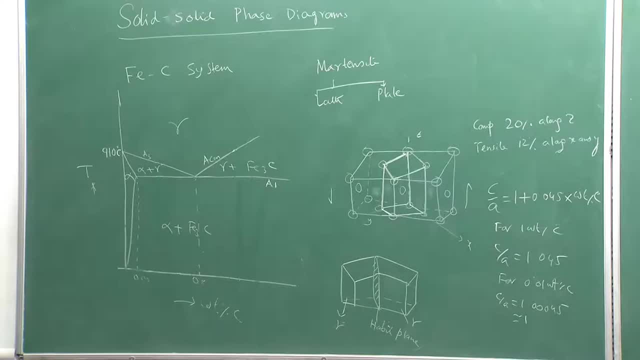 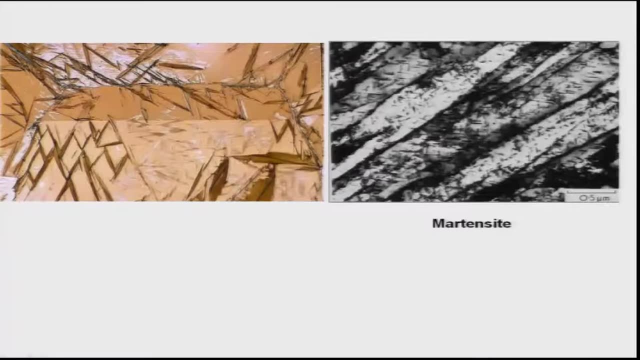 And this morphology will depend on what kind of steel you are looking at it, Like this one I showed you here. You see here. these are the plates in this picture. This is optical microgram which I am showing you here. You can see here. these are the prior gamma grains: 1,, 2,, 3,, 4, 5, 5 gamma grains. 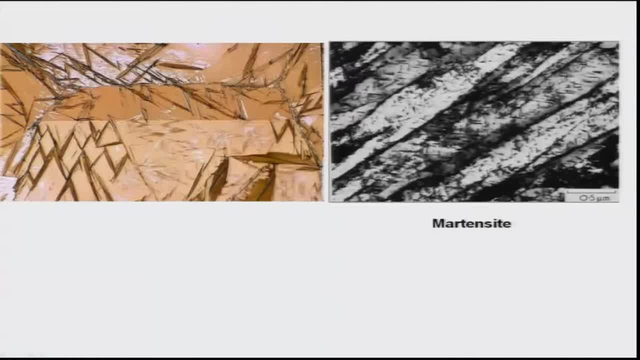 You can even see the boundaries and the martensites have formed like a tree bunch or leaves of a tree. They are actually called lats. They are called lats. They are called lats. Lats are martensite. On the other hand, here you see, they are plates of martensites. 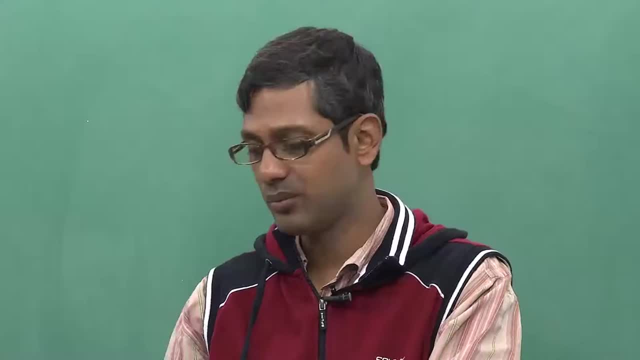 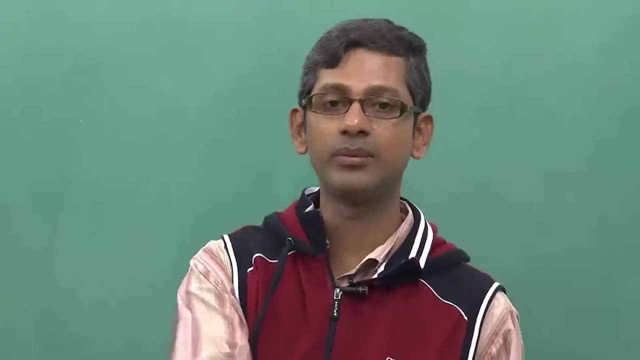 So these are the two typical morphology of martensites. So in the next class we will discuss more on martensites and I will tell you the basic theories behind it, of martensite, because martensite transformation is very important for the steel. metallurgy. Thank you.